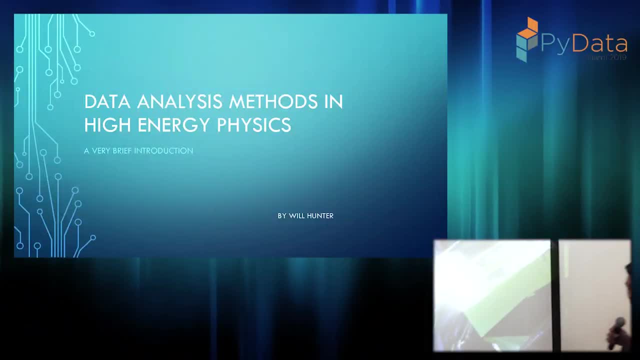 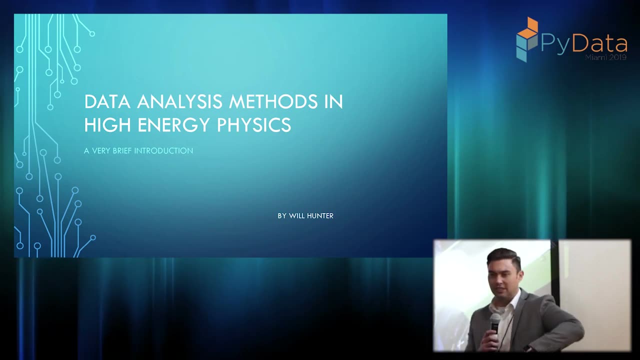 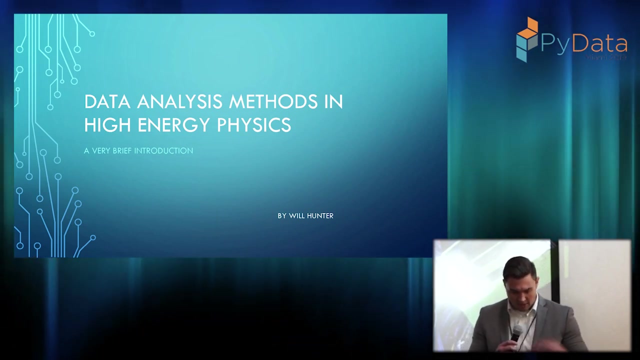 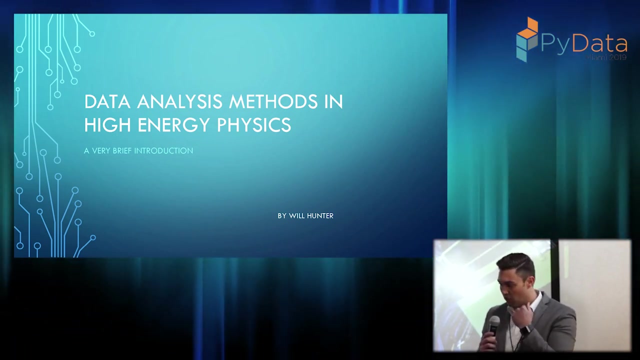 Hello. So we'll see how this talk goes, because I don't know how the rabbit hole for like particle physics goes pretty deep. Yeah, fantastic. I saw the quantum generalized models. I was like if it weren't right before I would have been in there watching along. Yeah, so. 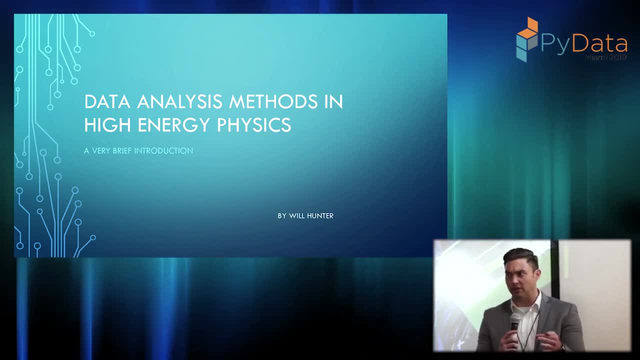 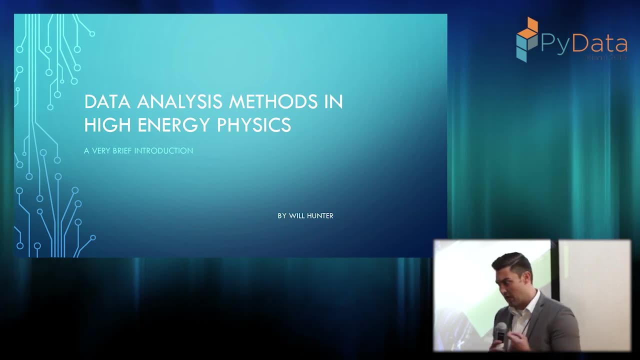 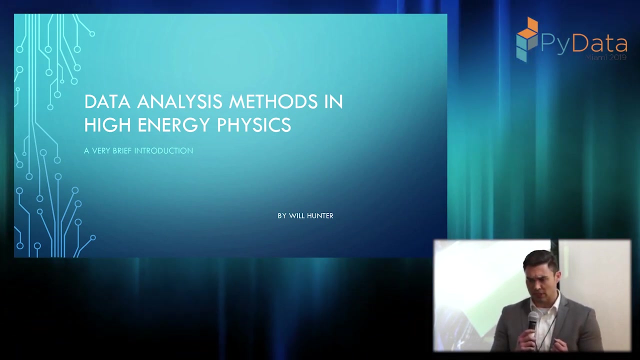 the first part of this presentation is going to be a very brief introduction to the standard model, Just showing you guys the particles And then, depending on how much time we have left- because that's freaking awesome, by the way- we can actually get into actual data. 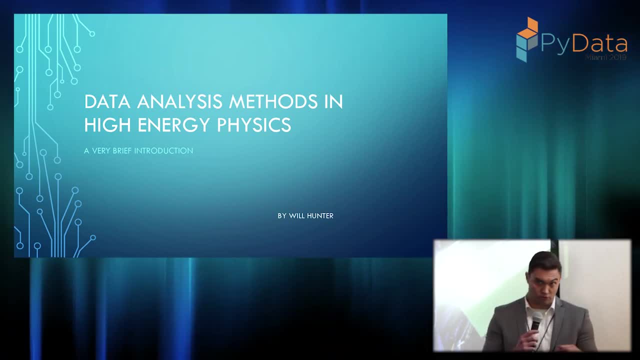 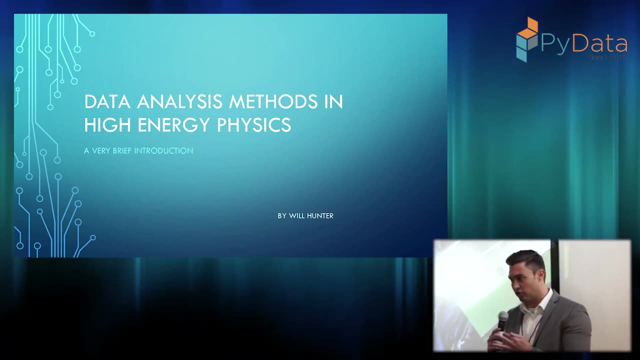 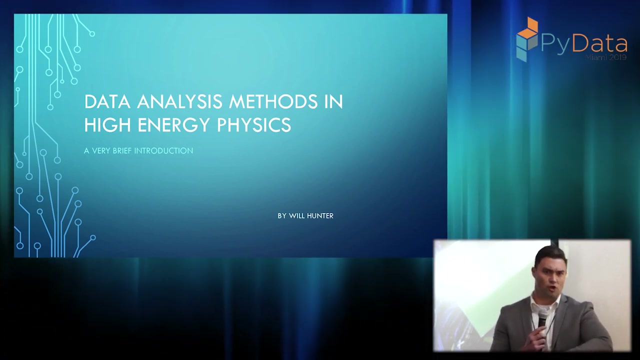 analysis Like: what cuts did you make on data in order to calculate the mass of, like, the Z boson? Hopefully we have more questions. I'm going to try to leave a lot of question time because that way I'll know what's actually valuable to you guys, as opposed to hey, here's all the information I've ever collected about. 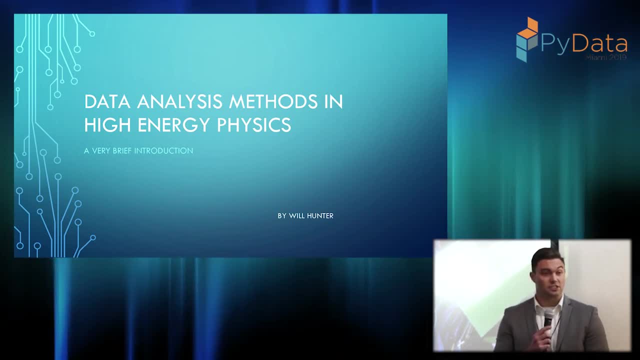 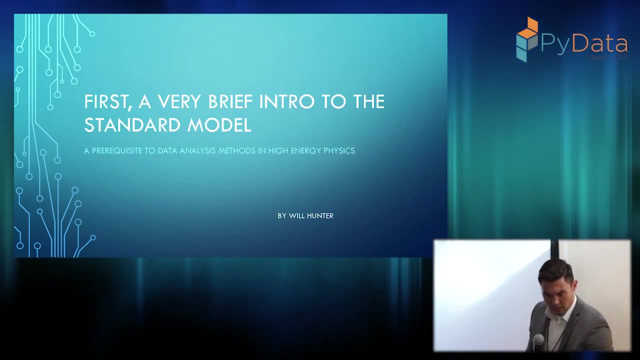 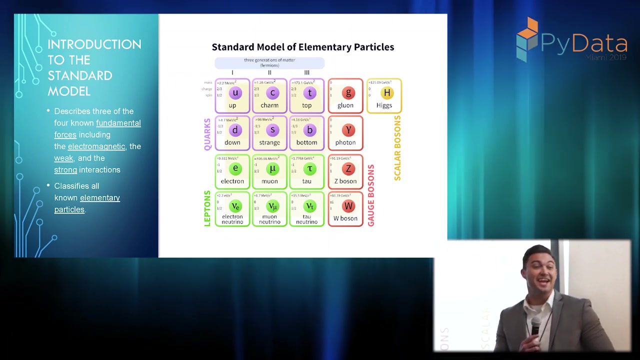 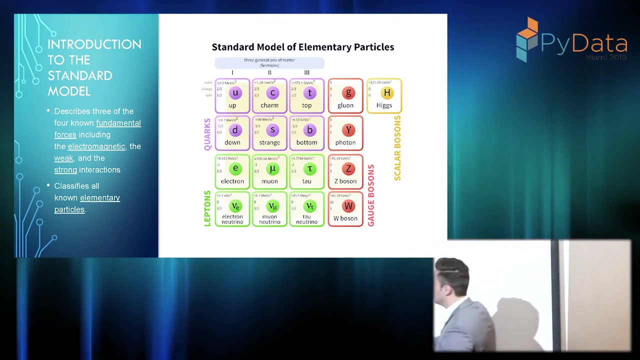 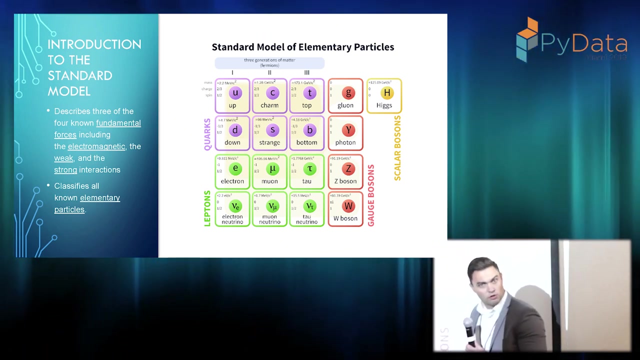 this stuff, Okay, Fantastic. Thank you guys all for being here, by the way. So how many people have seen this before? Yeah, You have a lot of energy. That's good. That's good, Okay. So most of matter is made up of these particles and electrons. Here you have your force mediators. 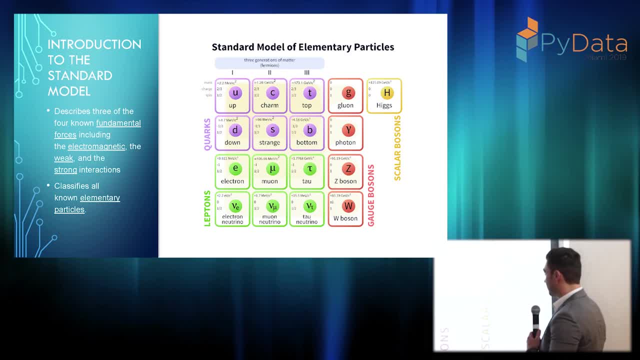 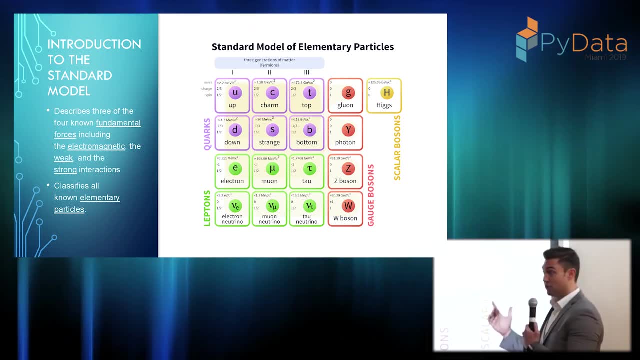 And here's the Higgs boson. I don't have time today to describe why we need the Higgs boson, the Higgs fields, But after this talk, we can talk about that too. You don't have to memorize any of this stuff. I will say that. 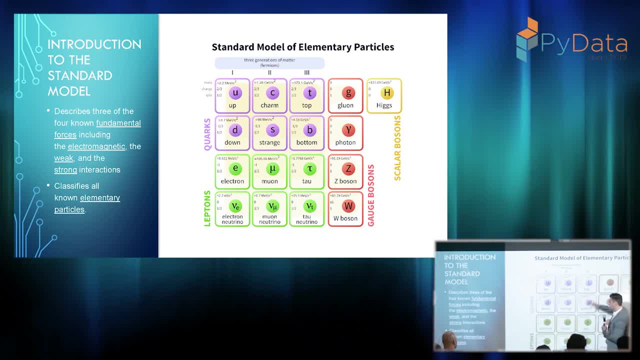 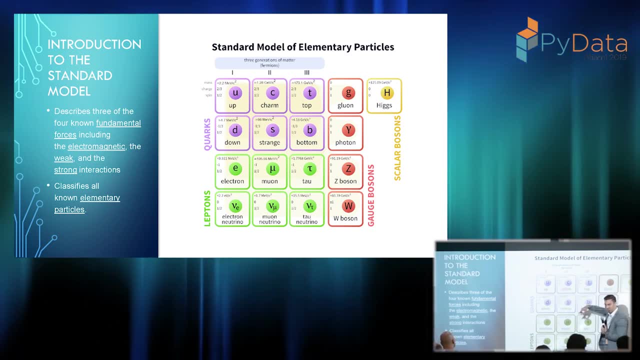 the muon is the only particle that you probably didn't use in like a chemistry class or something like that. They will be discussed today. Up and down, quarks make up protons and neutrons, And you guys know about electrons, Okay. 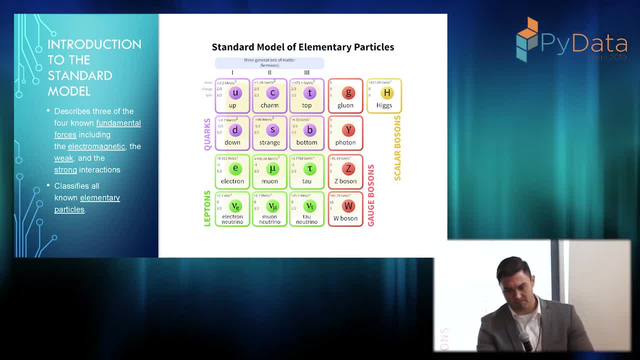 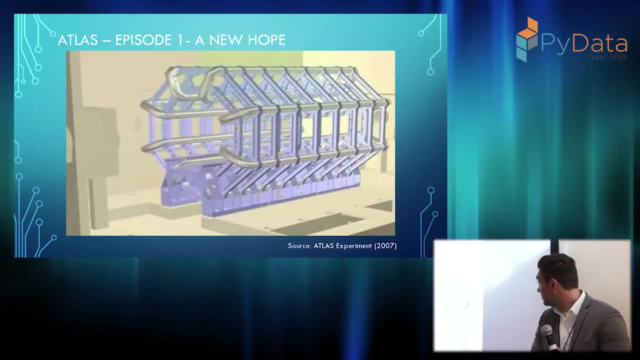 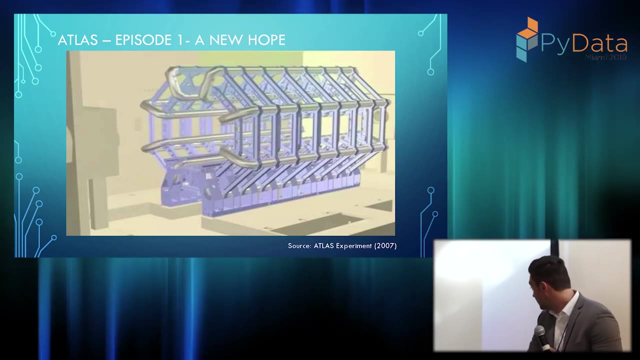 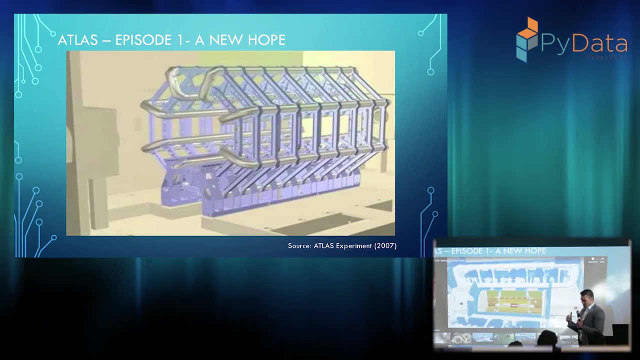 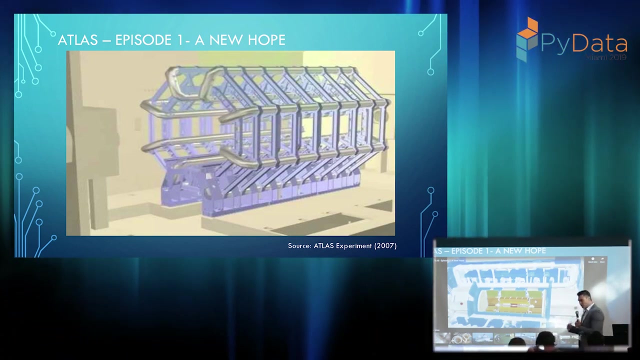 Let's see if it's worse. Yeah, videos are awesome. Visualization has really helped. Okay, I should also probably talk a couple of things. In order to find these very, very small particles, we smash like 10 to the 10th protons going like 99% speed of light. You can see particles that haven't existed. 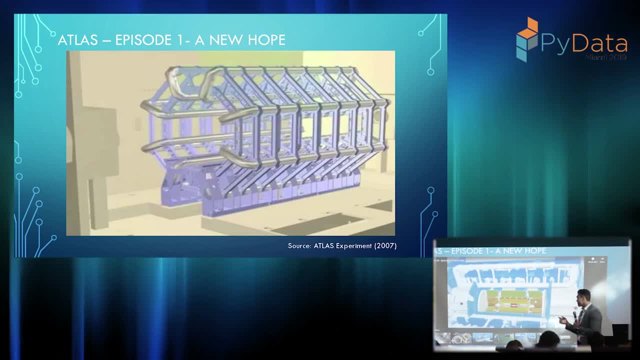 since like the beginning of the universe. There's a how many people here have heard of the LHC large Hadron Clarion? There's a how many people here have heard of the LHC large Hadron Clarion? Wait a minute. how many people here have heard of the LHC large Hadron Clarion? 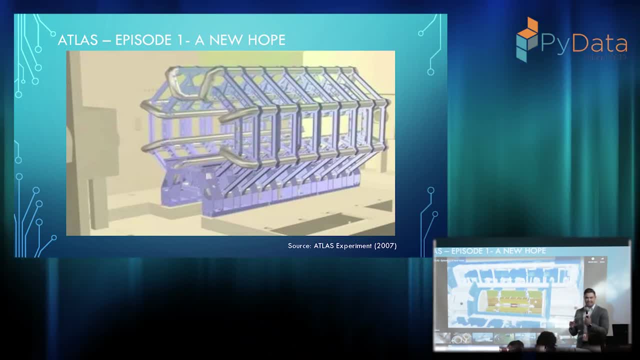 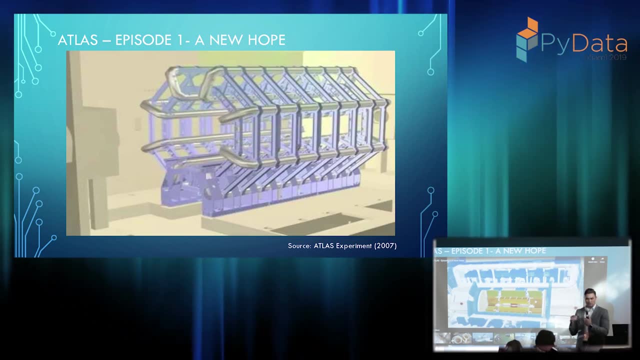 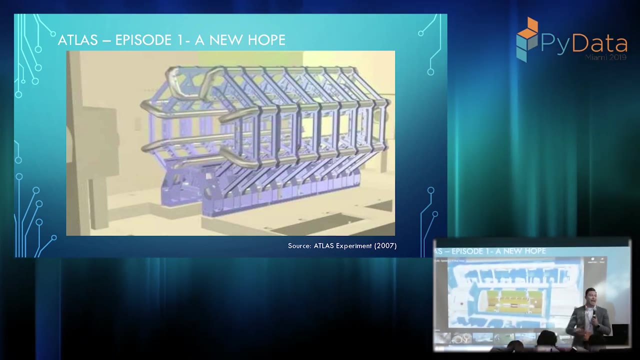 Hadron Collider: Nice, nice. When I'm amongst nerds, I feel like I'm amongst friends. How many people here know what a Hadron is? Fair enough, fair enough. So Hadrons were made of the cork material. but I have you here so I'm like: do I talk about mesons? No, not today. So there's a. 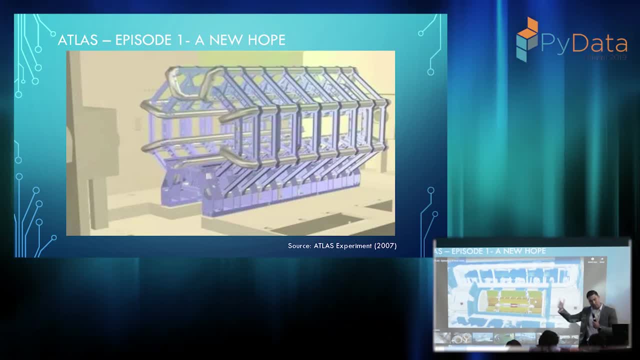 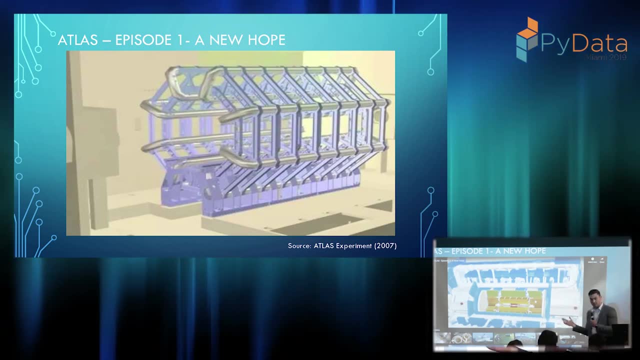 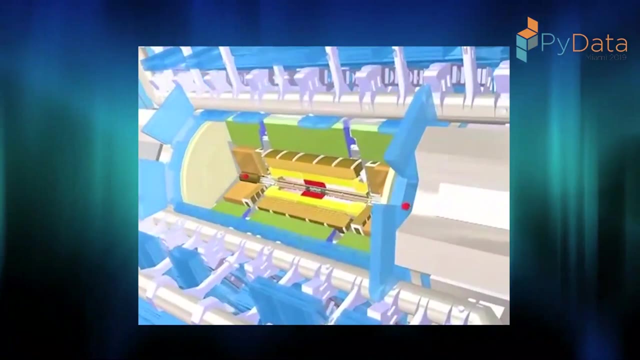 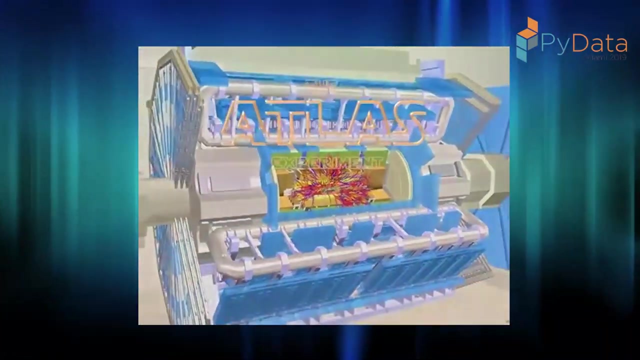 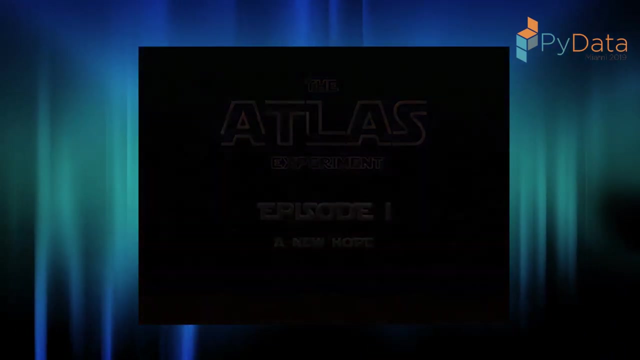 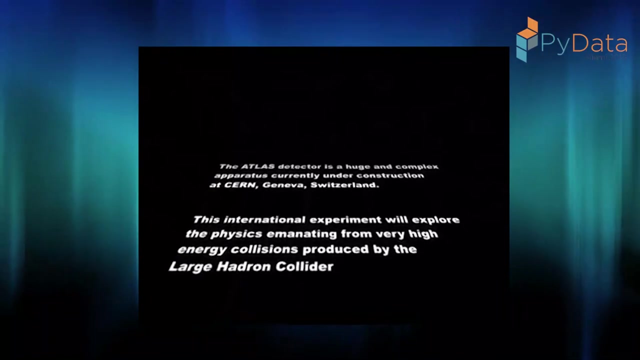 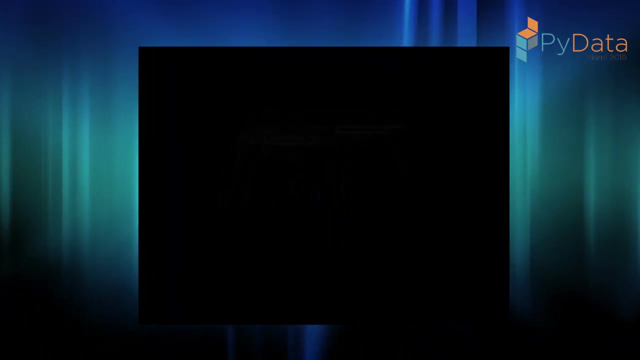 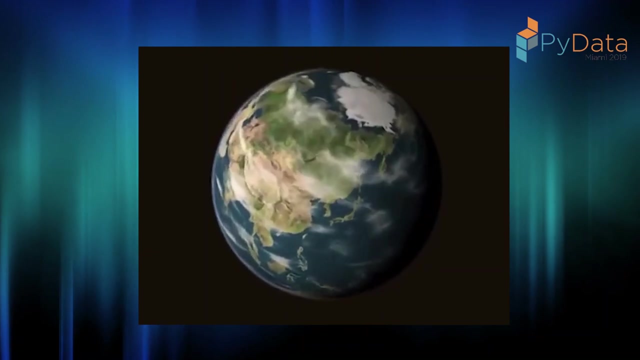 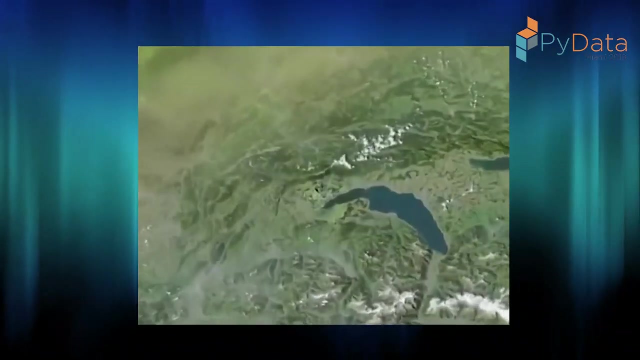 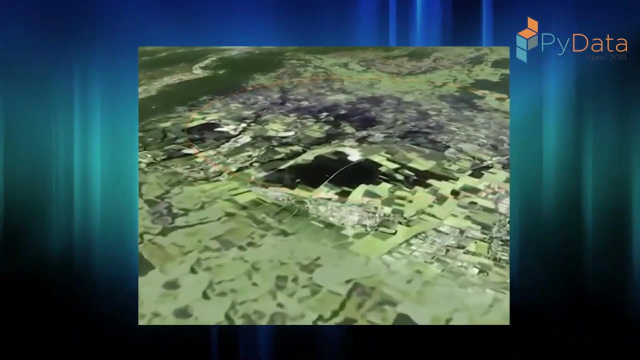 couple different experiments that are going on at CERN and the LHC, and the one that I actually did data analysis with was from Atlas, So this explains Atlas better than I could. So in a 27 kilometer underground ring near Geneva, protons are accelerated to near the speed of. 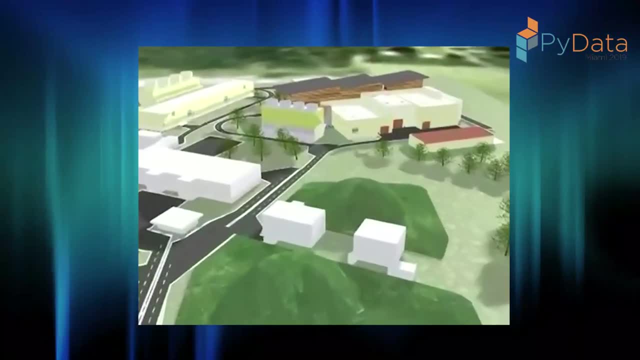 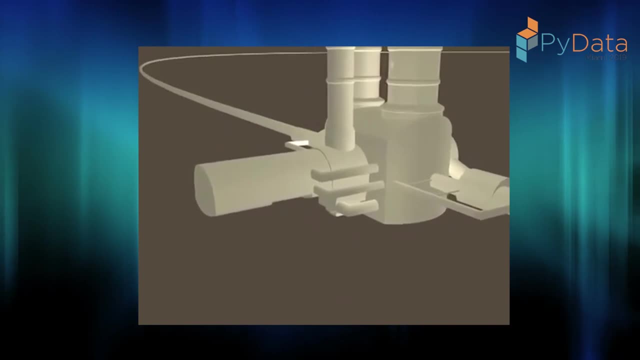 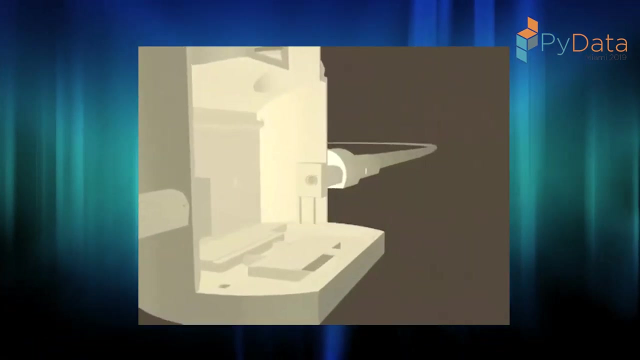 light and collided Here at the CERN laboratory. scientists can recreate the conditions of the universe immediately after the Big Bang. The huge Atlas detector which studies these collisions took several years to assemble, but through animation we can watch it in a few minutes. 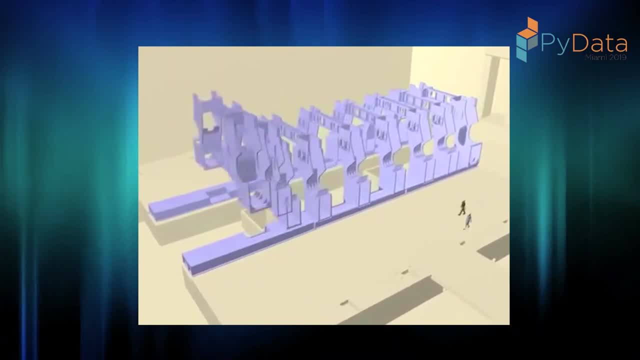 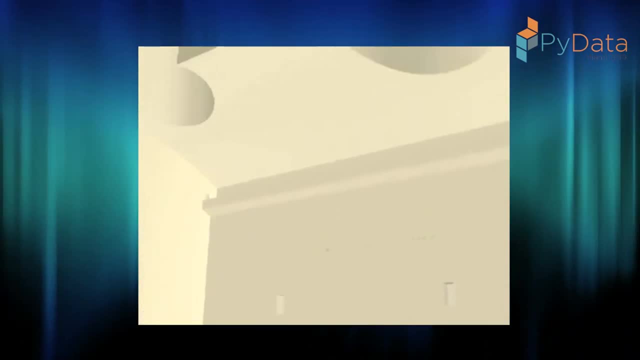 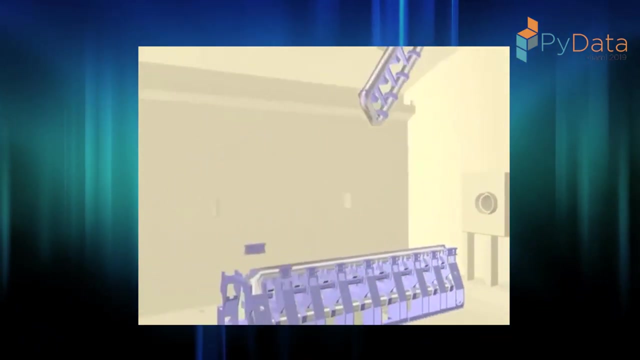 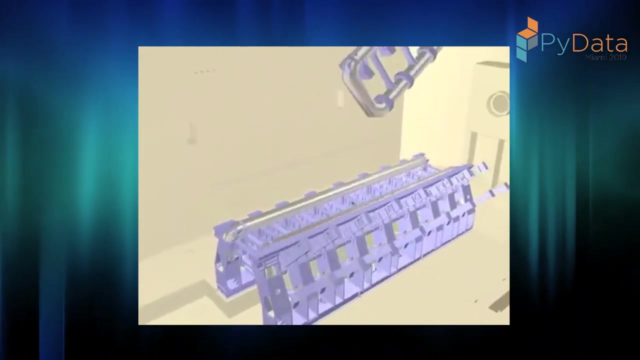 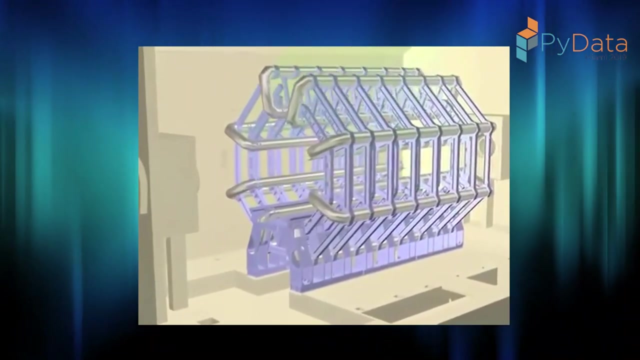 Throughout much of the Atlas detector there is an intense magnetic field. This is produced by passing current through about 80 kilometers of superconducting cables housed within a large toroidal structure. This enables Atlas to maintain one of the world's largest volumes of intense magnetic field. It is important to measure the energies of particles which pass. 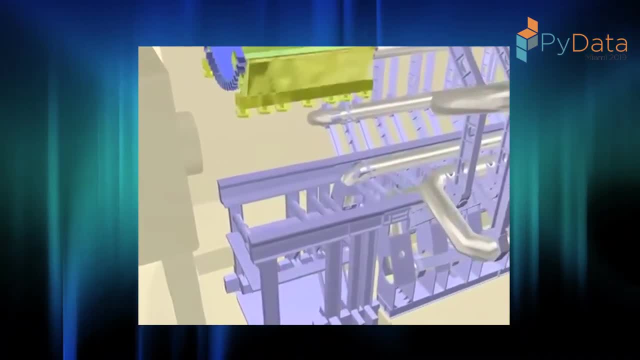 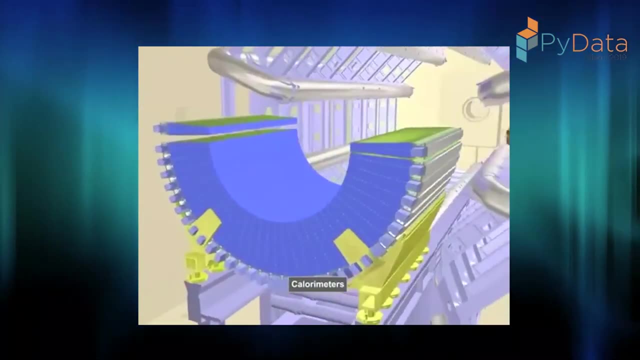 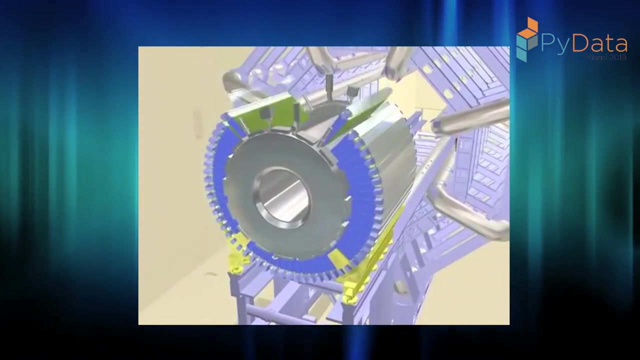 through the detector. This is done by a device known as a calorimeter. Atlas has several types, which are arranged as barrels placed in both the center and at the ends of the detector. The 3,000 ton tile calorimeter is composed of steel and a special material which lights up when particles. 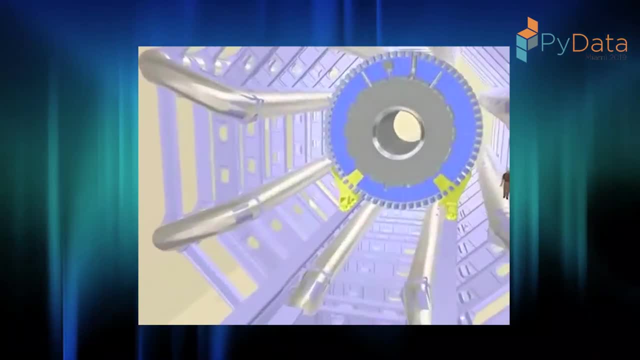 pass through The tile. calorimeter is a special material that is used to measure the energy of particles in the atmosphere. The higher you measure, the less energy you hidden there. A total of 1300,000ol is measured per calorimeter. The 3,000 ton calorimeter surrounds a second. 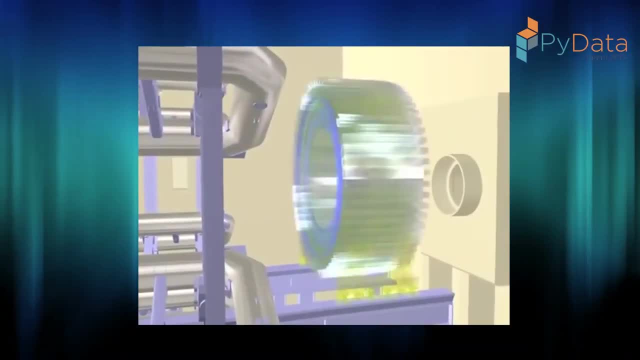 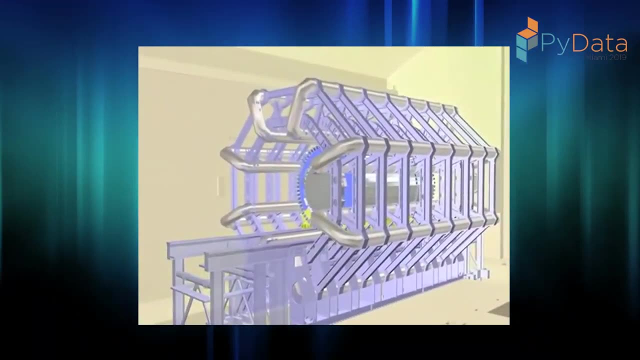 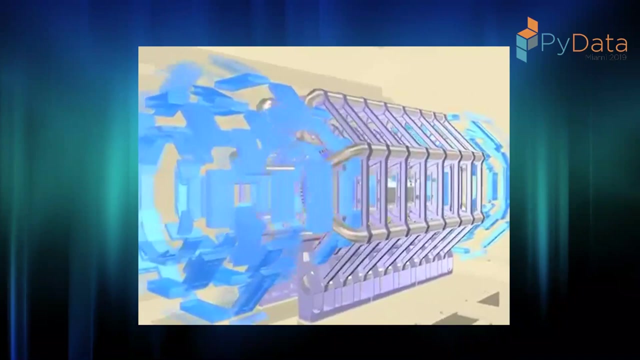 calorimeter, which consists of lead bathed in liquid argon, which is cooled to minus 180 degrees Celsius. This is known as the electromagnetic calorimeter. Outside of the calorimeter, there is a further component which measures the trajectory of charged particles, called muons, that reach the 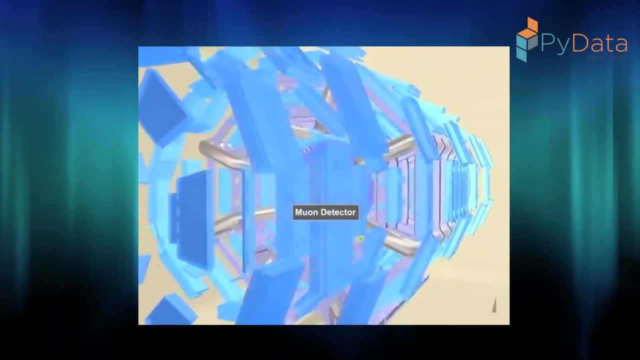 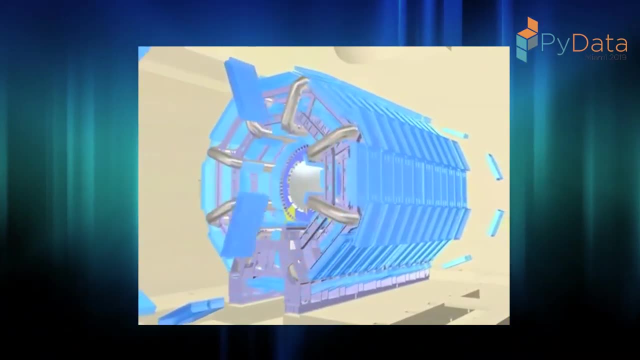 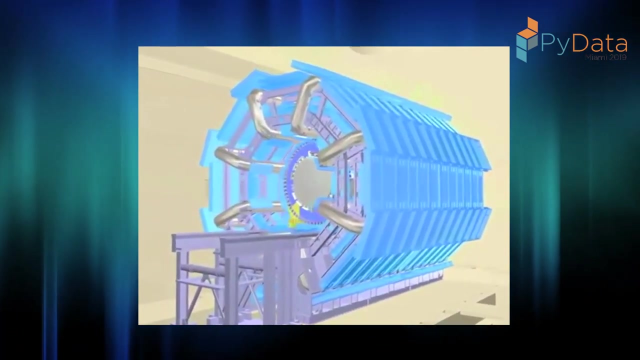 outermost layers. The surface area of this component, the muon detector, is around the outside of the is around the size of several football fields close to the heart of the detector. several components are designed to measure the trajectories of passing charged particles with an accuracy of close to 1 hundredth of a millimeter one. 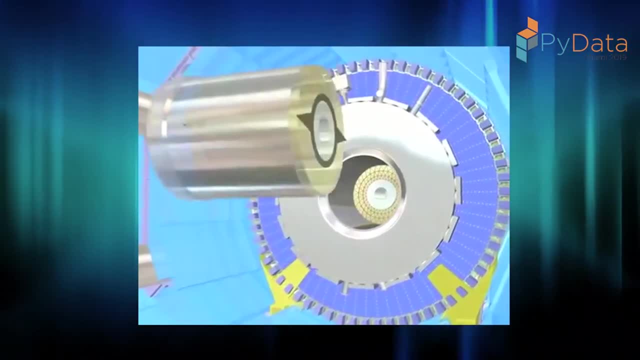 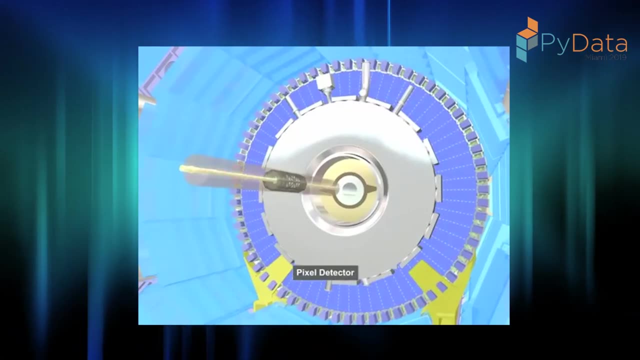 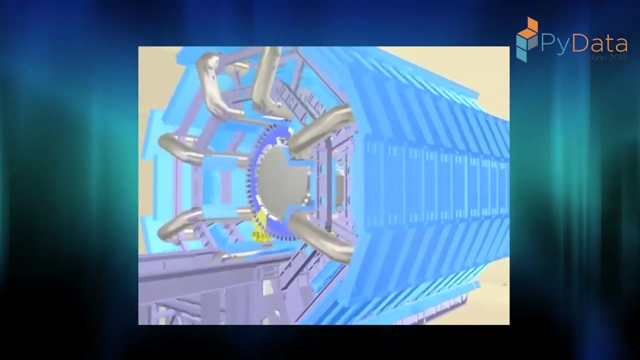 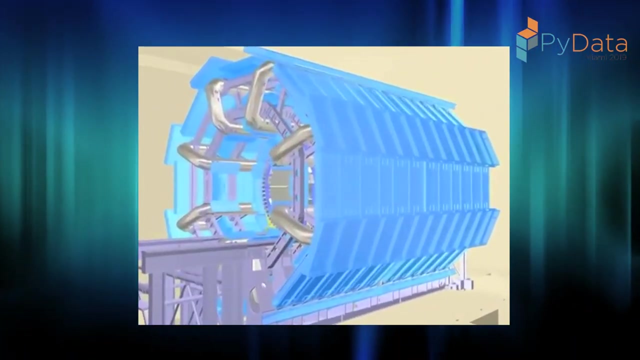 component, known as the transition radiation tracker, consists of several hundred thousand tubes filled with gas and gold wires. inside the transition radiation tracker are several detectors built out of silicon and divided into millions of thin strips and tiny pixels. the Atlas detector is designed to measure as many particles as possible. 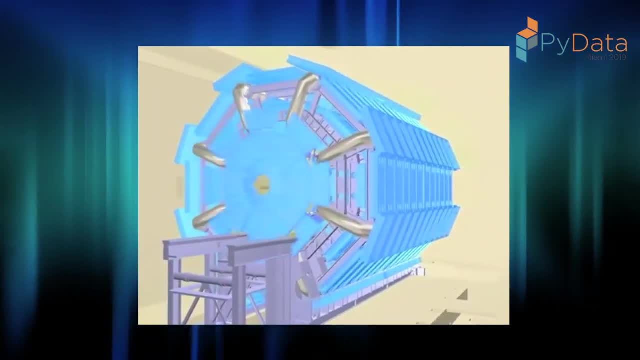 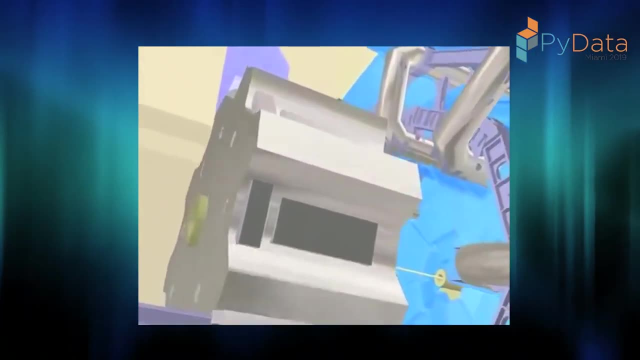 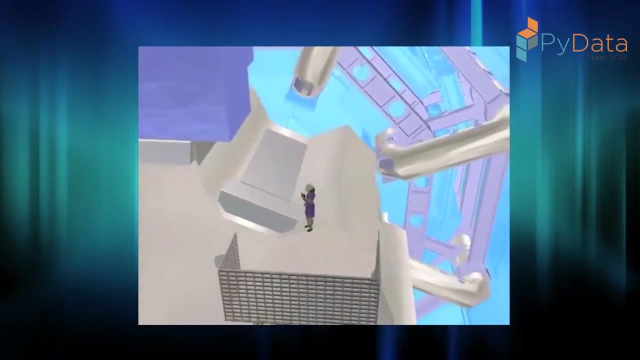 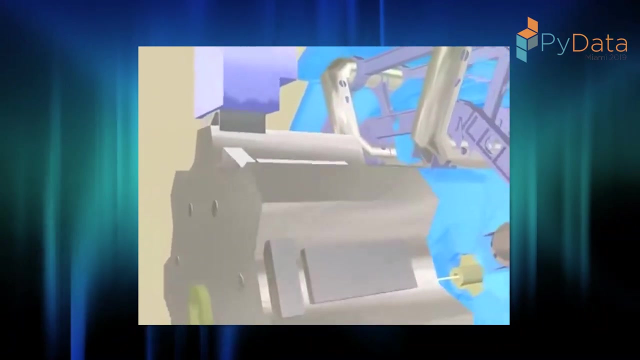 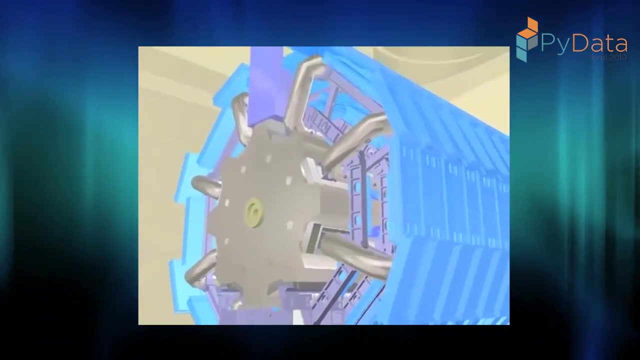 and further. detector modules are placed at the ends to measure particles produced at small angles to the proton beams. toroidal magnets are placed at both ends of the detector to produce the intense magnetic fields that Atlas needs you. the detector is a completely new technology and can't possibly see water. 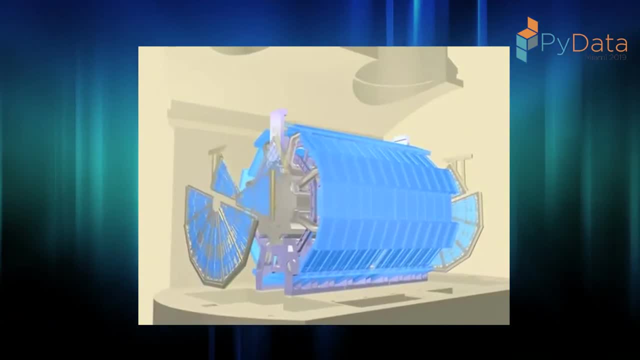 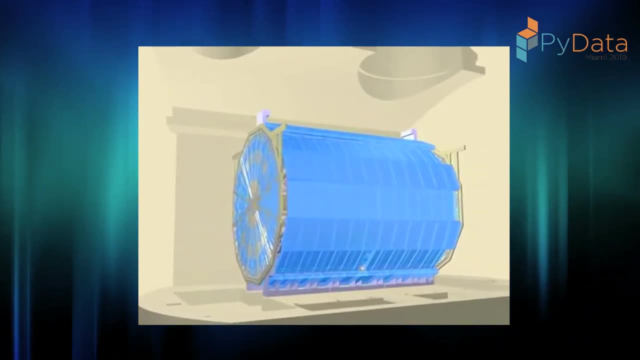 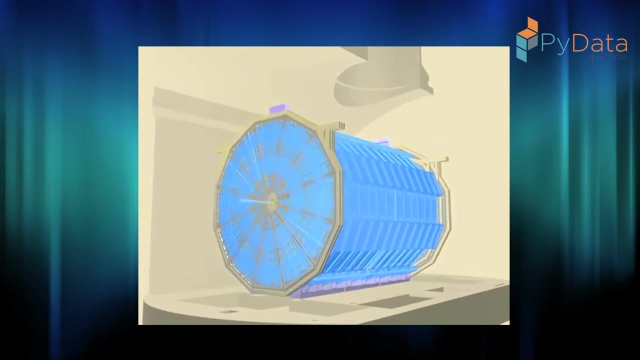 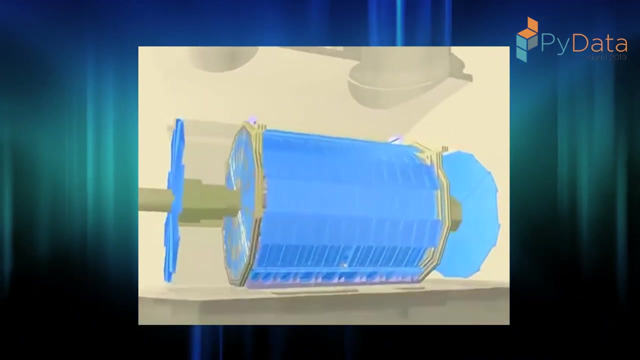 the detector is a completely new technology and can't possibly see water. the detector is a completely new technology and can't possibly see water. The detector construction is finished with the addition of further layers of detectors for measuring particles which reach the edges of ATLAS. Now let's look inside the detector. 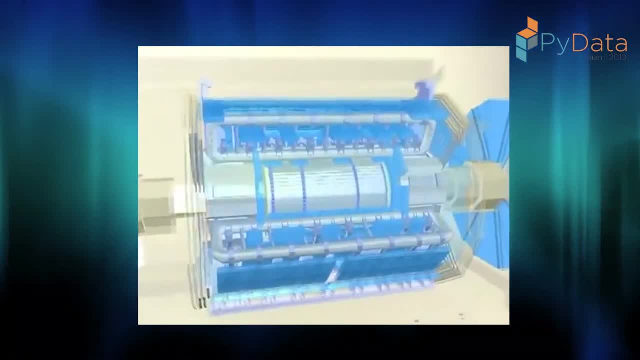 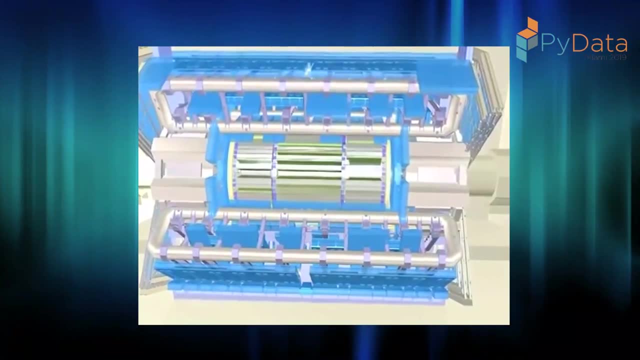 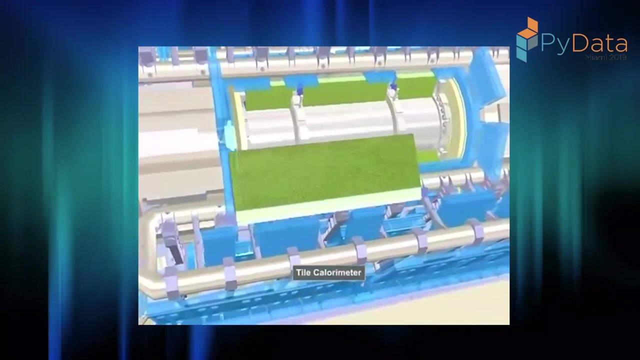 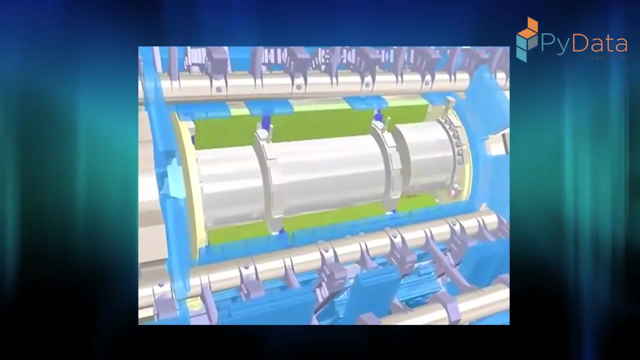 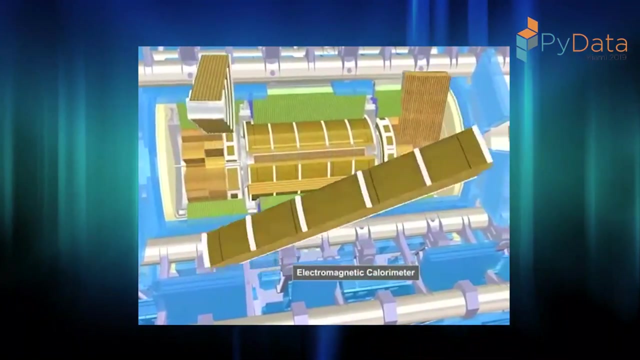 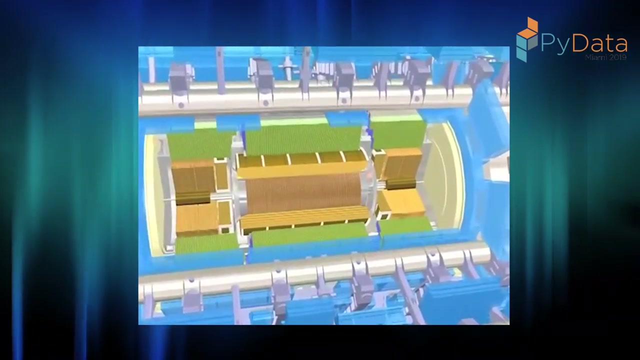 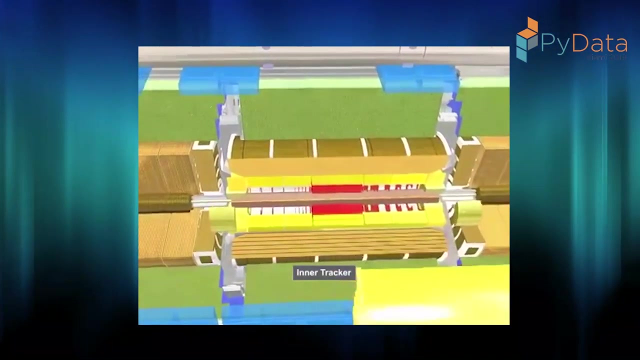 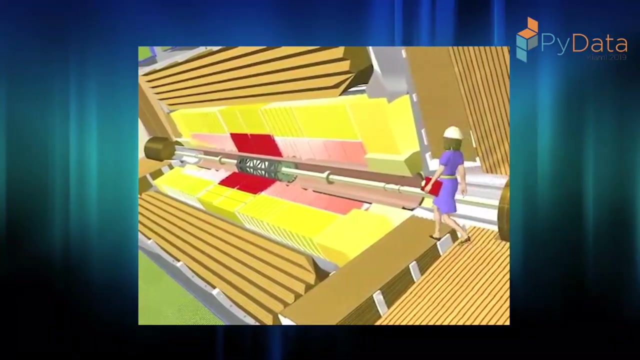 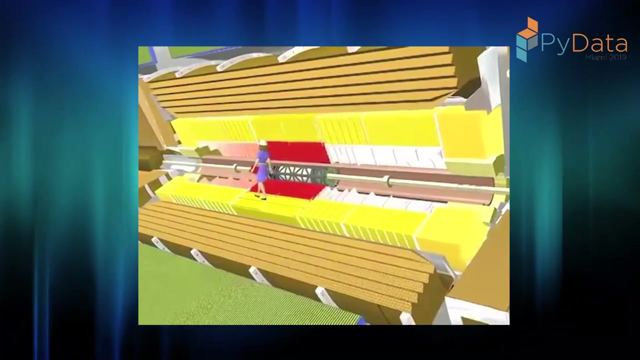 Here we can see in more detail the pieces of individual components: the tile calorimeter, the electromagnetic calorimeter, the transition radiation tracker and the silicon devices. In reality, a scientist would not be allowed to walk through the open detector, but in this case it illustrates the sheer scale of the ATLAS detector. 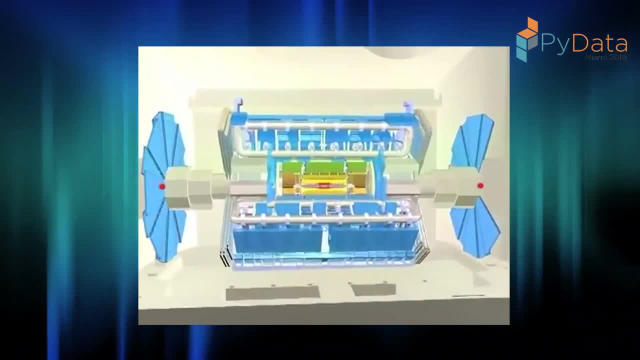 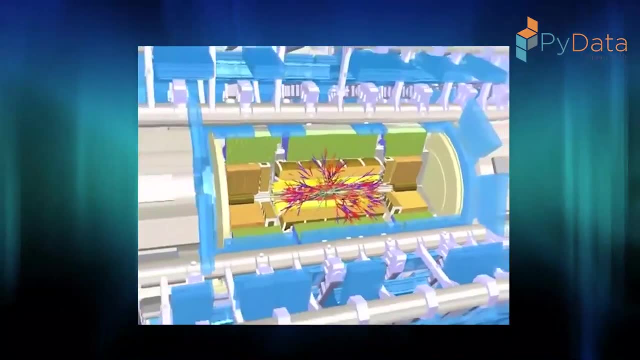 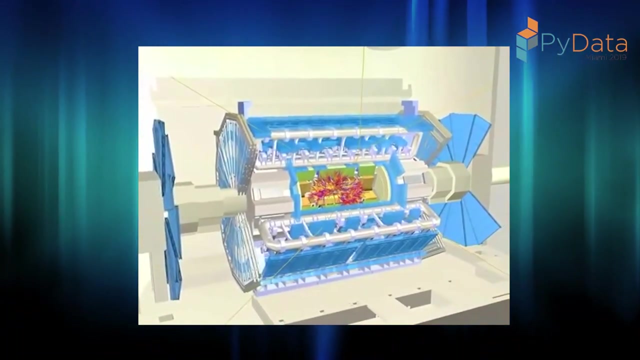 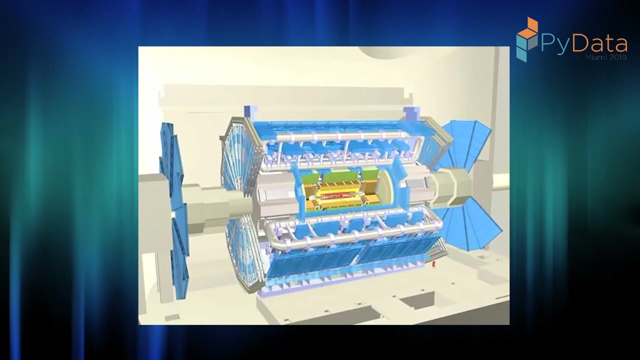 Now we can finally witness the ATLAS detector measuring the particles from the colliding protons. A typical collision produces many hundreds of particles, and each component of the ATLAS detector is necessary to build a full picture of the collision. If you want to know how it all works, don't miss Episode 2, The Particles Strike Back. 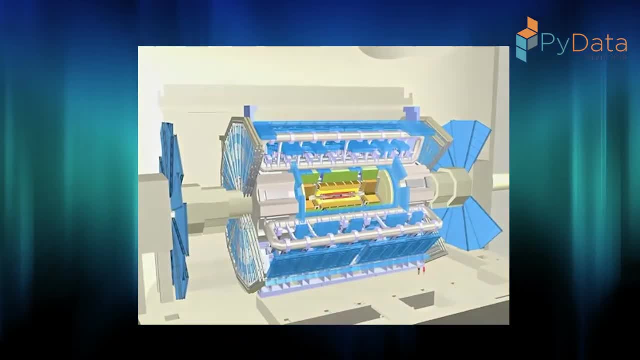 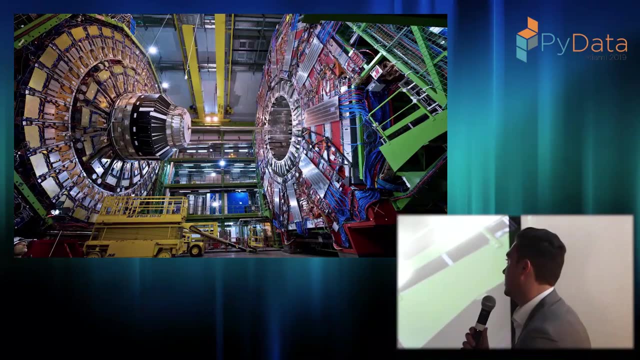 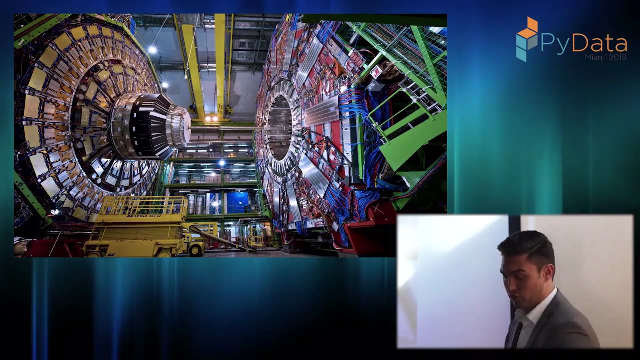 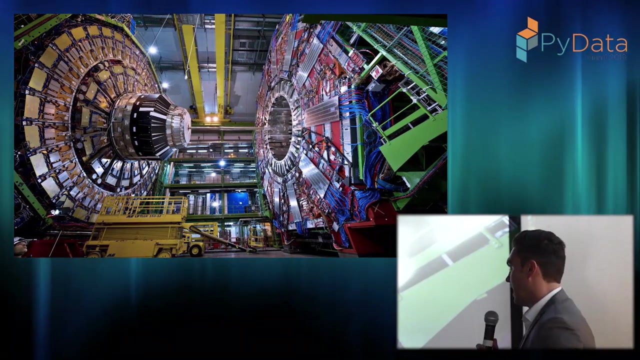 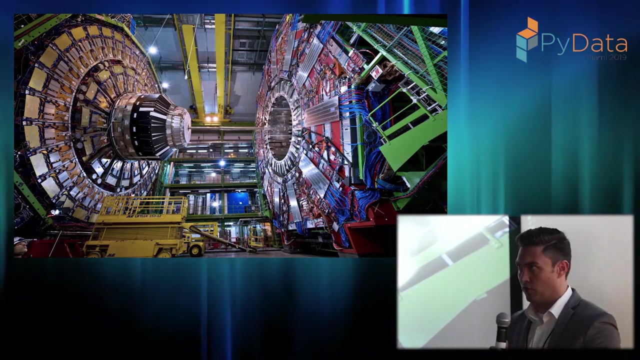 That was a pretty good model of it. This is what it looks like in real life, when it's, of course, not in use. So this thing generates a ridiculous amount of information every year, unlike the petabyte level, The. The next short video you'll see basically describes how they collect the data. 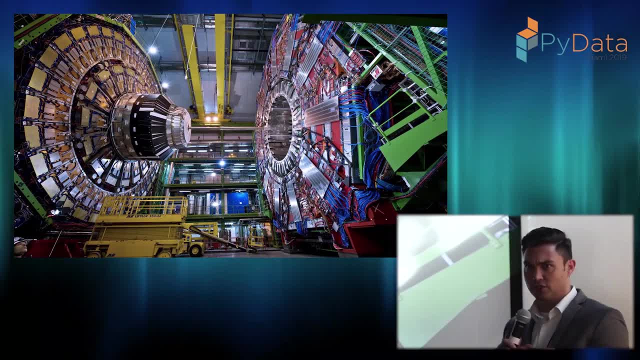 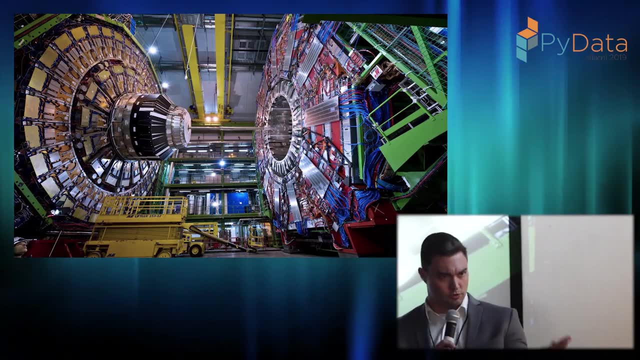 and how they kind of ship that around the world. Most of the stuff that I interacted with was not experimental data, it was the Monte Carlo stuff, so you can check like, hey, this is what my theory says we should get. 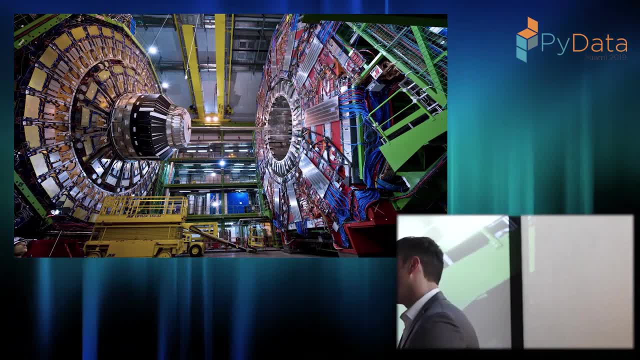 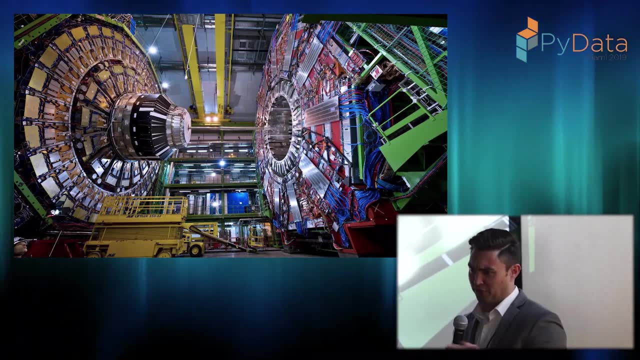 What did the experiment say When the Large Hadron Collider was broken down for a number of years it took a lot of like PhDs who were writing papers like extra years longer because it was broken. That kind of sucks. 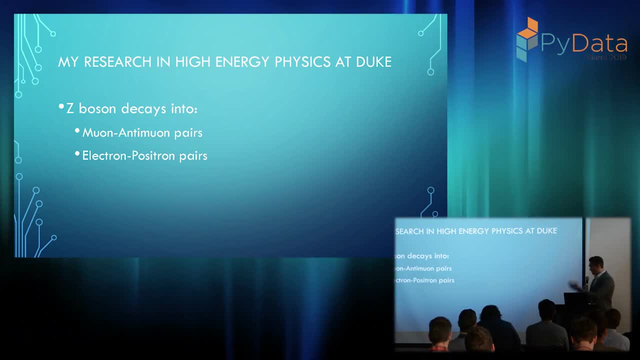 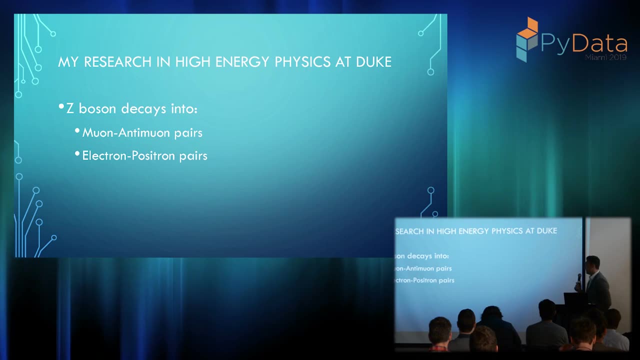 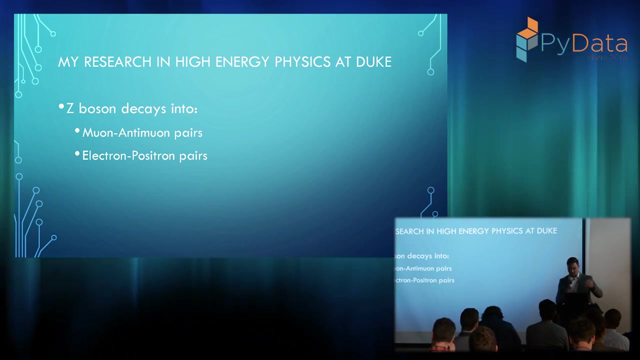 and it took 48 years before it could actually get tested and confirmed that the particle existed. That's a good run for funding stuff. So what particles can we see? We can see electrons. Well, I say: see Like we can detect electrons, protons and muons. 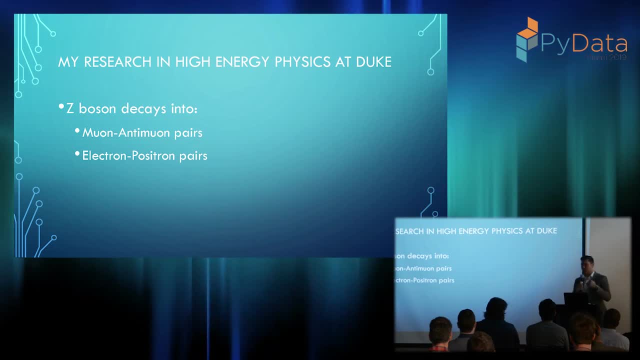 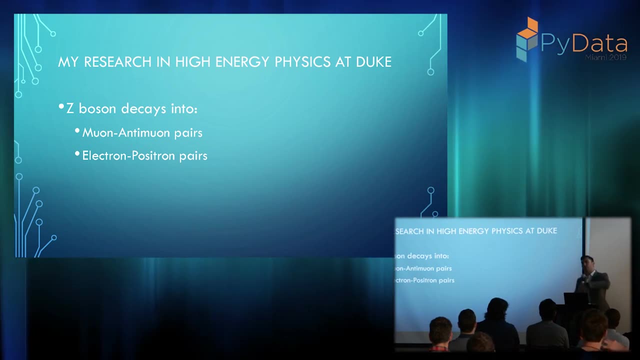 So what is a muon? A muon is like an electron, but it's roughly 200 times heavier. It doesn't live very long, but if you get them to go faster because of special relativity, it thinks that it's living the same amount of time. 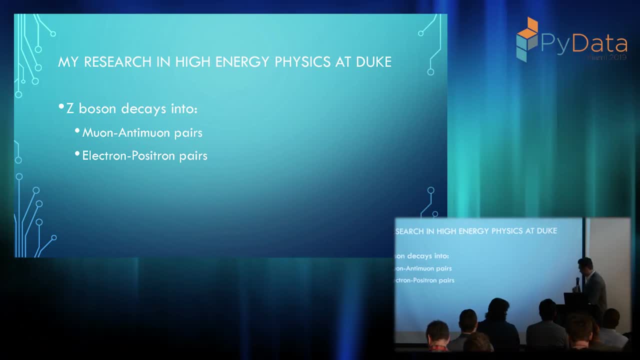 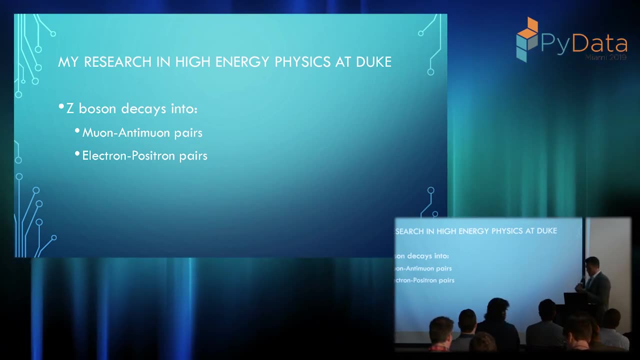 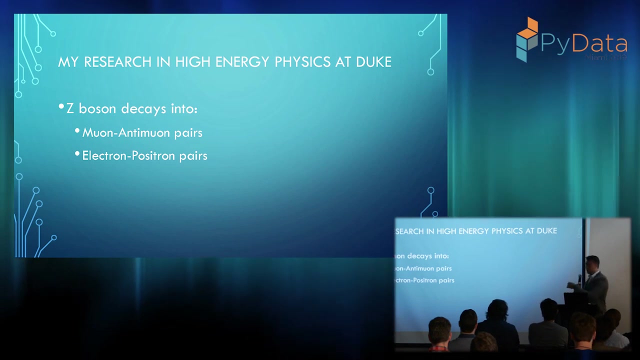 So you can get it to go as fast as possible. If it's a distance that's longer, then you can predict without special relativity. That's kind of cool. When a Z boson decays, two of its decay modes are into muon-anti-muon pairs. 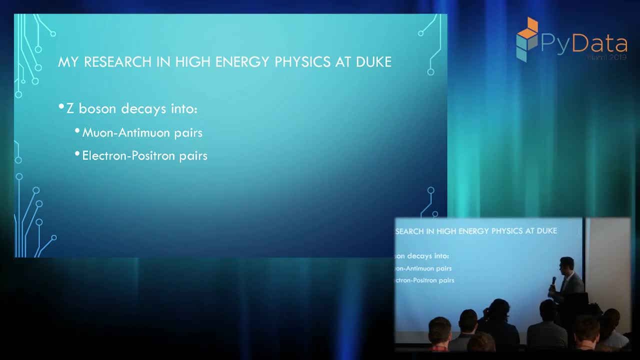 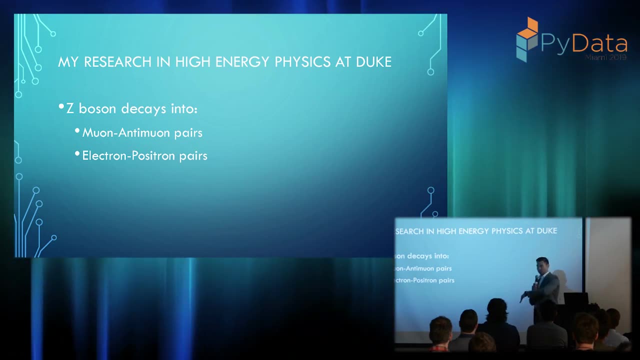 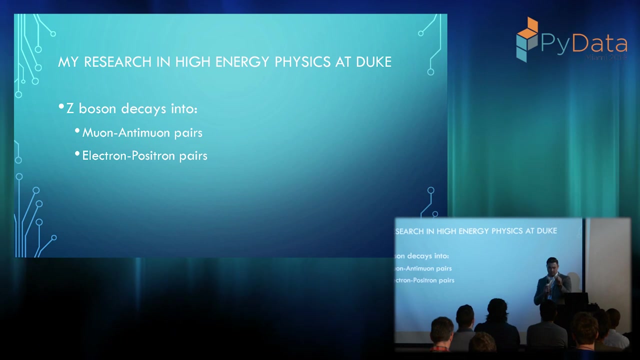 And so if you see one particle going off in this direction and you see another particle going off in exactly the opposite direction, when this starts happening like thousands of times, eventually you can't ignore it. There must be something there. One analogy that was used is like: 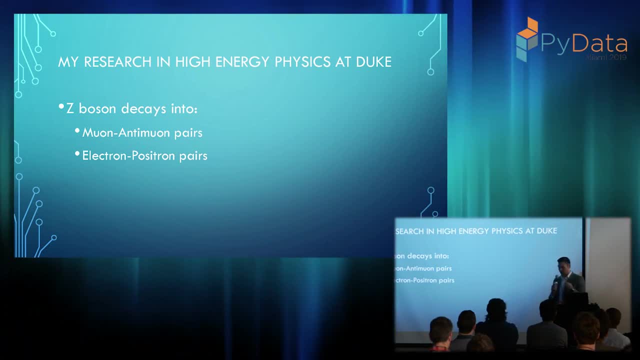 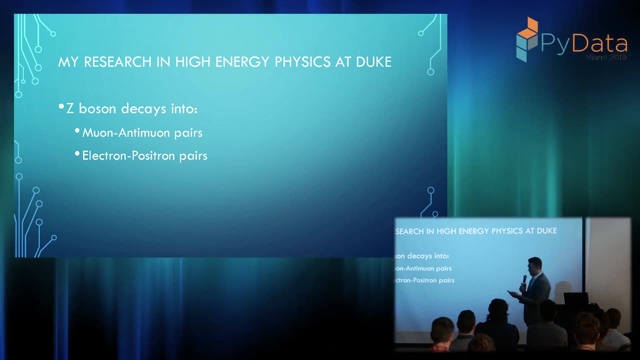 if there were an alien race that came to Earth and they couldn't see patterns of black and white, if they saw a soccer match at first, they'd be like what are they doing? And they might think that people are just running around in a field. 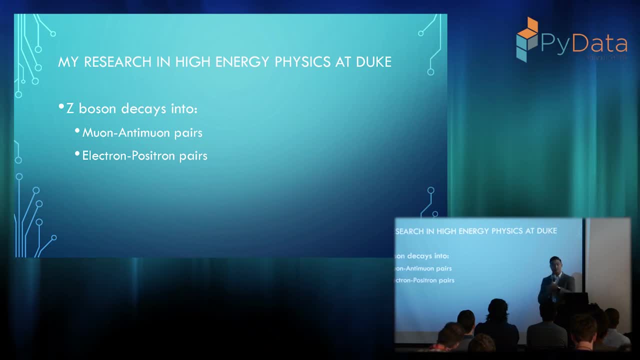 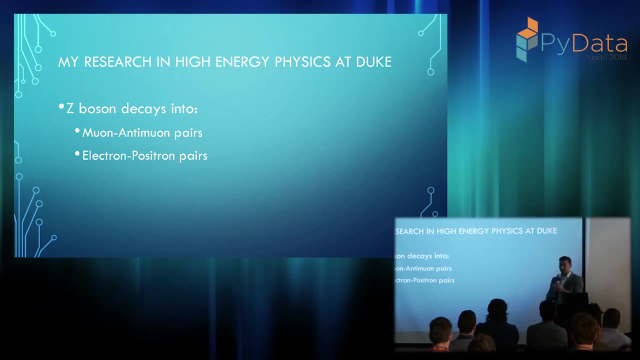 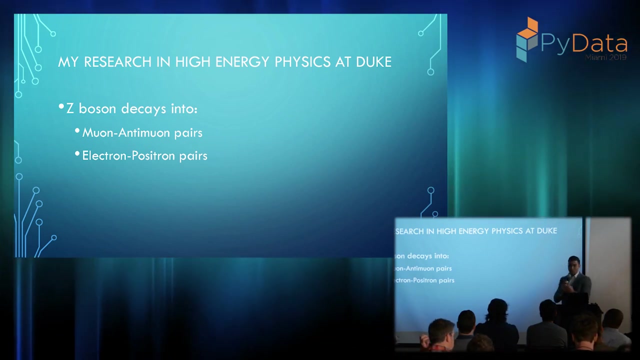 But eventually they might conclude that there's some ball, some particle that they just simply cannot see but still exists. That's how things like the Z boson and all the other particles of the standard model that we can't see directly, that's how we know they're there. 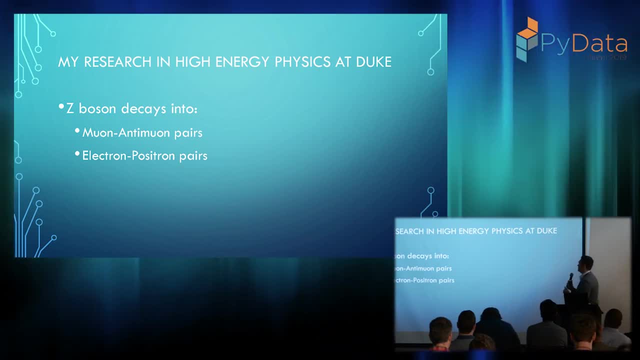 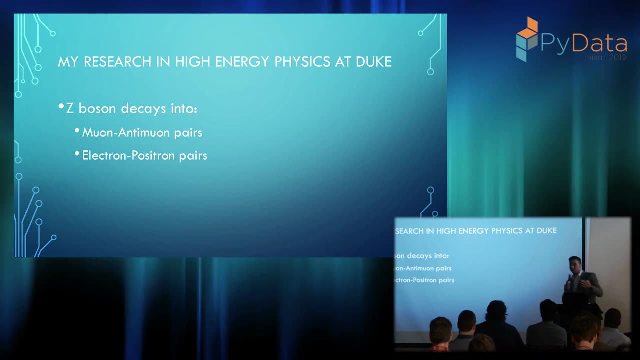 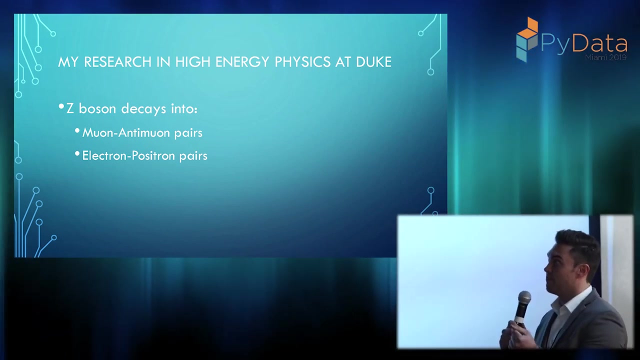 because we've done this millions of times. Now, why do we care about the Z boson? We care about the Z boson because the Higgs boson is predicted to decay into into a pair of Z bosons. So if we can see enough pairs of Z bosons, 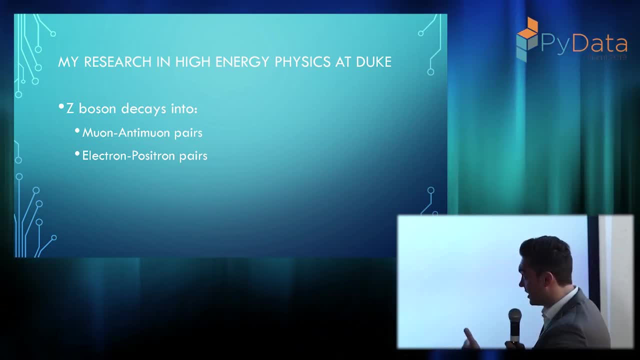 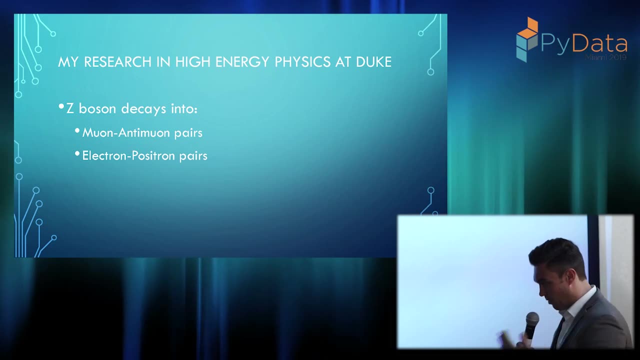 well then something, some particle is there. Perhaps it's the Higgs, perhaps it's not. That's Now. we're pretty confident it is the Higgs particle, But you have to run it through a bunch of other tests before you say okay. 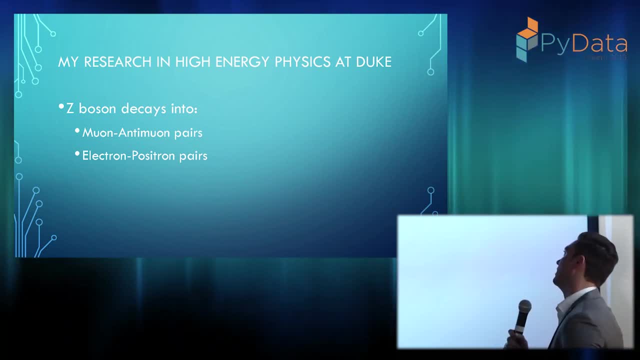 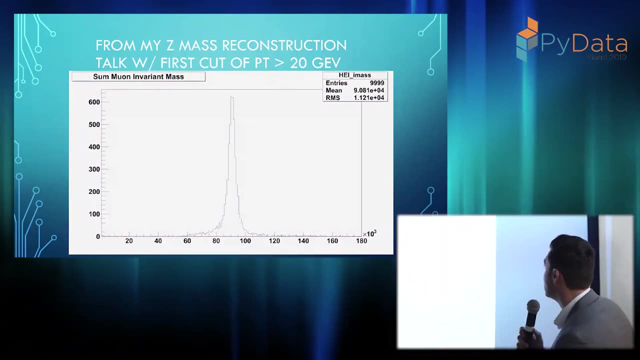 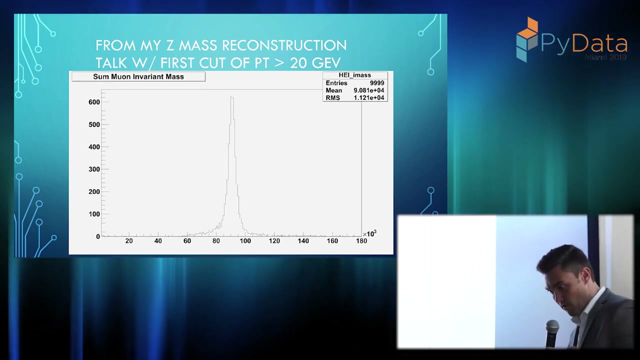 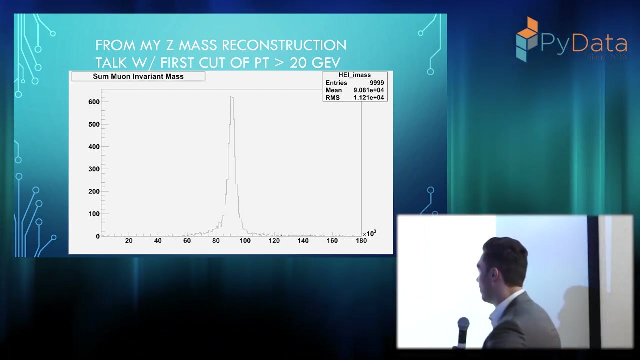 this is the Higgs boson that was predicted by those theories. So So You generate monochromatic data. In my case, you get it from CERN, from one of those Tier 2 centers, And at first, like you, have a ton. 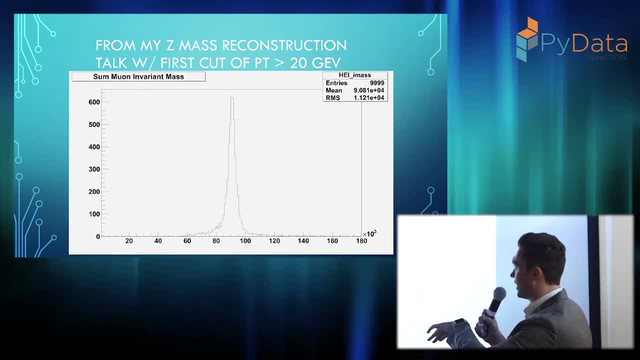 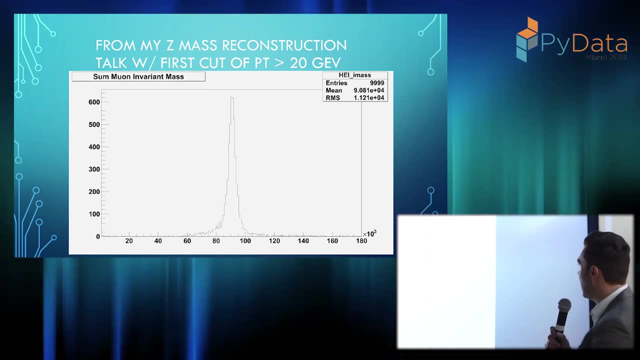 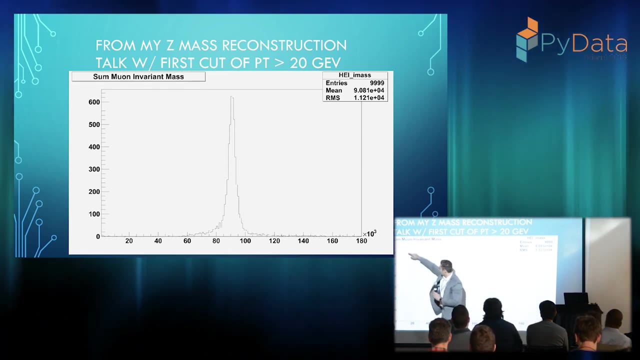 This is after some of my selection cuts. A lot of them have like no energy or like null events, And so usually this peak looks like down here And then you have like a big bucket- that's like you know- over here. 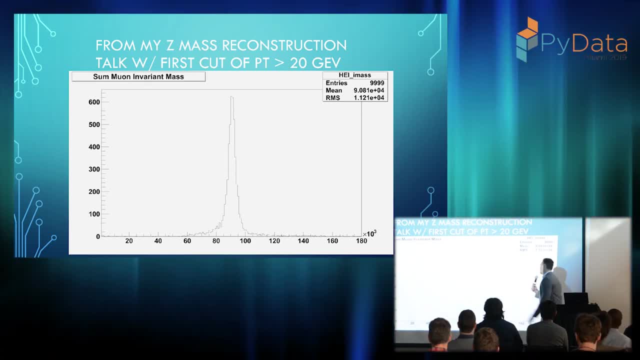 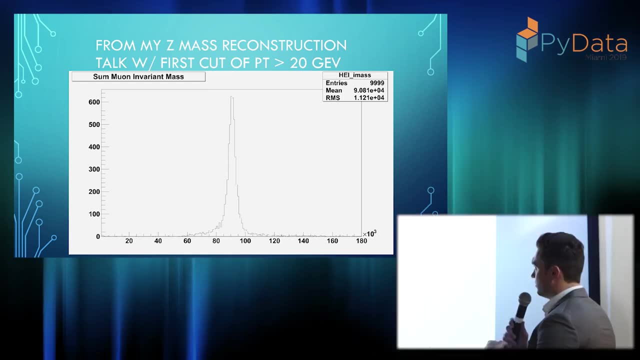 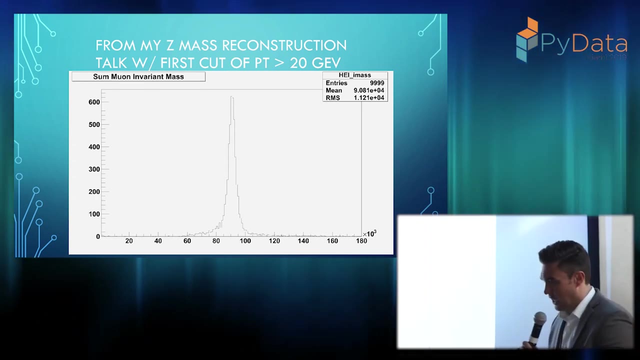 You cut those out because it doesn't make your graph look pretty. And uh, Then you want. You want higher energy. Your data looks better when you go for higher energy particles. Um, In order to say how you calculate the invariant mass: 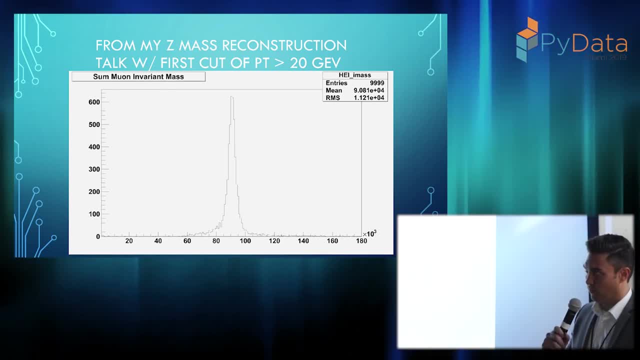 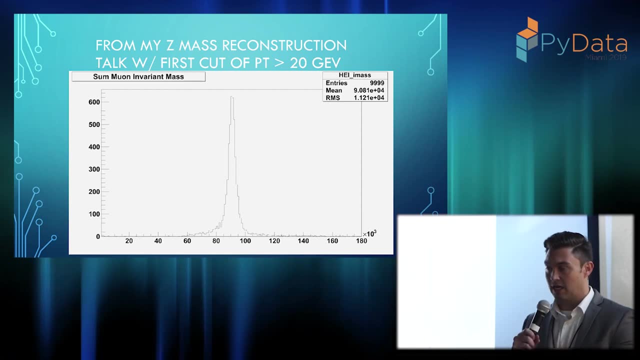 or what is the, What is the invariant mass? I would have to write out: Uh, Have you guys? So you guys know, like E equals MC, squared for that. Well, it's not the complete. It's not the complete story. 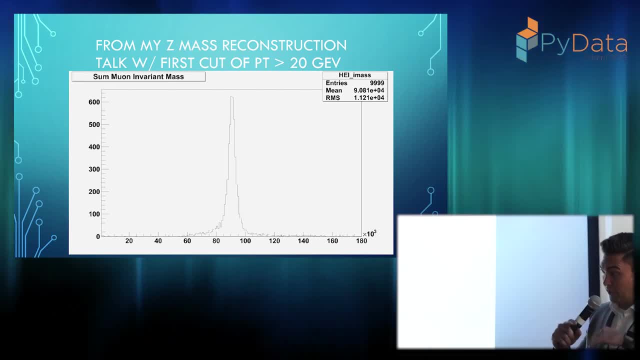 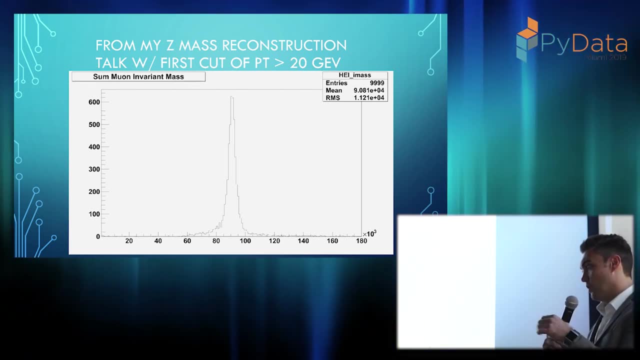 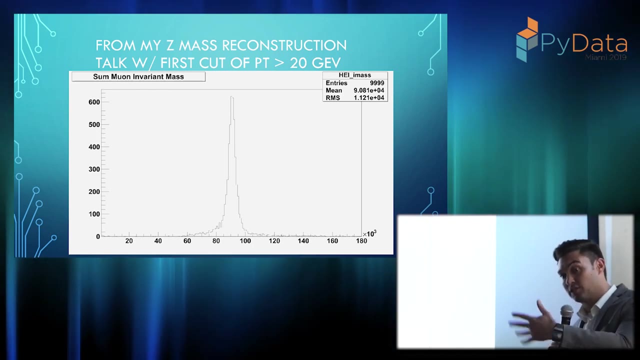 It's actually: E squared equals the MC squared, that quantity squared plus the quantity PC squared Um. When you subtract the That momentum side, Let's see if you have E squared. You subtract the That P squared side and you take the square root of that. 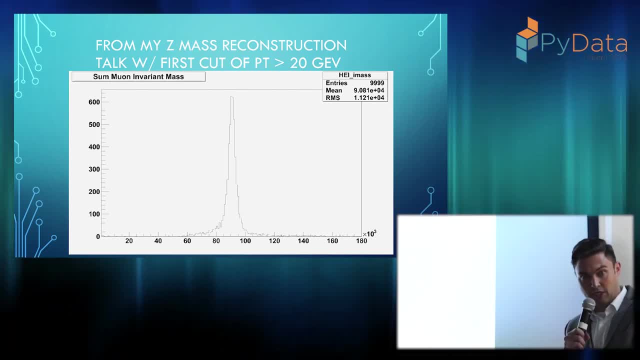 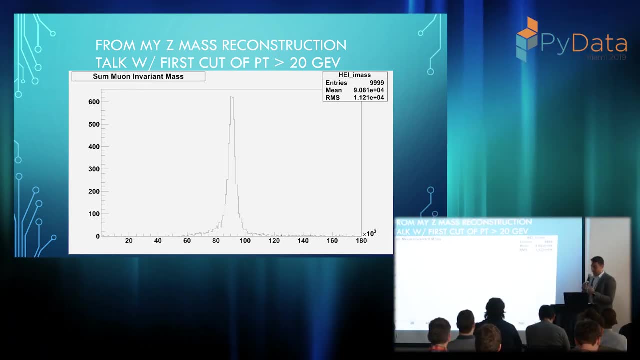 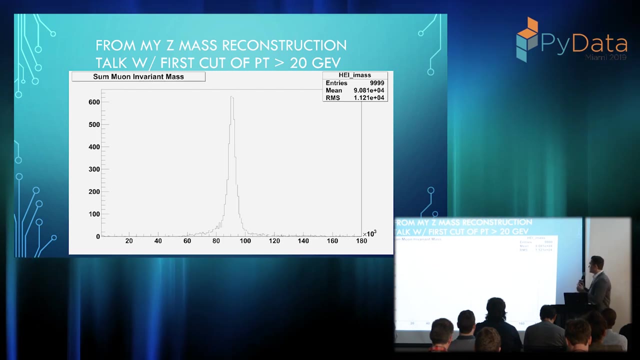 to find the invariant mass. And you say, Hey, does my distribution match what the physical theory tells us? Uh, And if? If your theory, If your theory doesn't match the experiment, usually you gotta go with the experiment. Um, 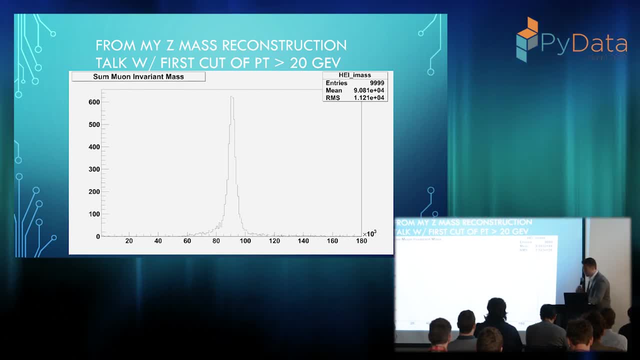 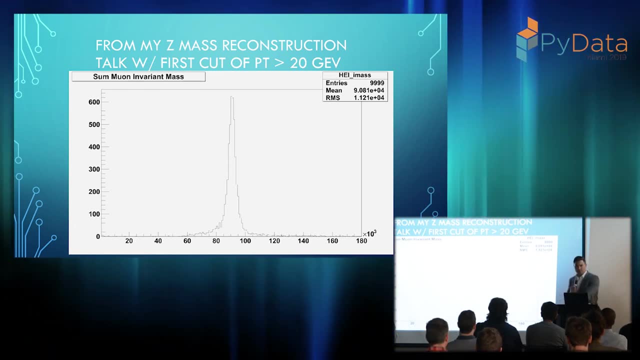 So, Anyway, There's five minutes left, so I'd rather take questions, because I don't know what you guys know and what you don't know. and that's very stressful for me, Uh, Because then I don't know what's valuable. 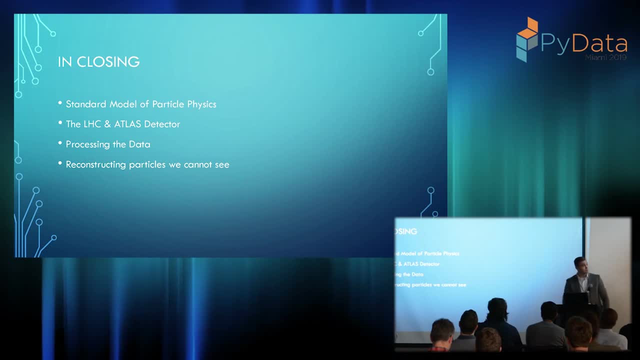 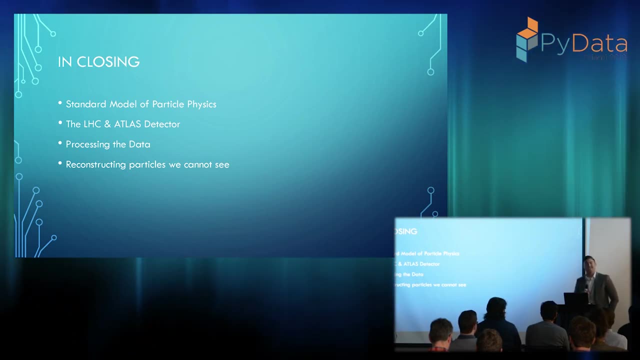 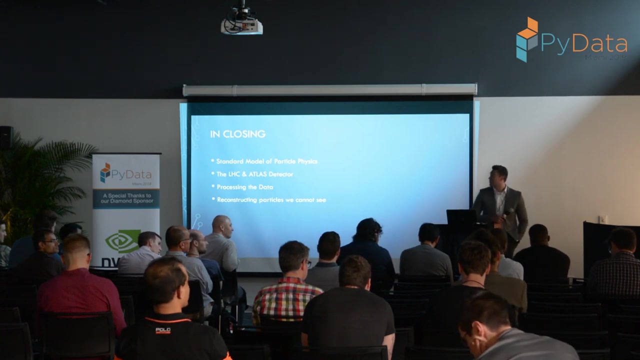 and what's not. So let's just go to that Questions. If you didn't clap, you're right, I ended. I'm kidding, Thank you. Thank you so much, That was really interesting. Um, I guess this is more along the line. 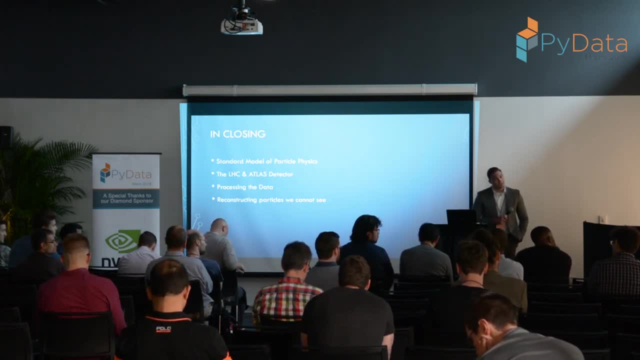 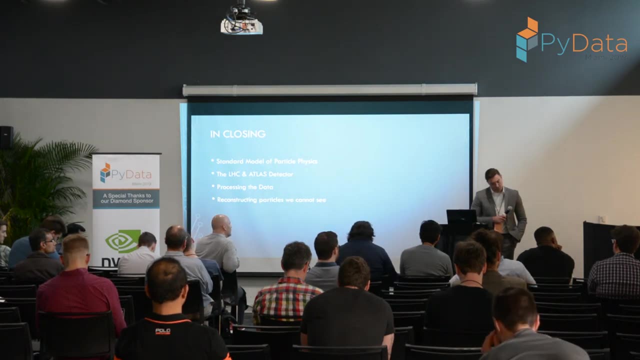 of kind of the selection of what you're looking at. What sorts of algorithms are you using when you simulate the standard model pieces that you want? Are you like doing a Bayesian method of within a tolerance or just kind of simulating things? 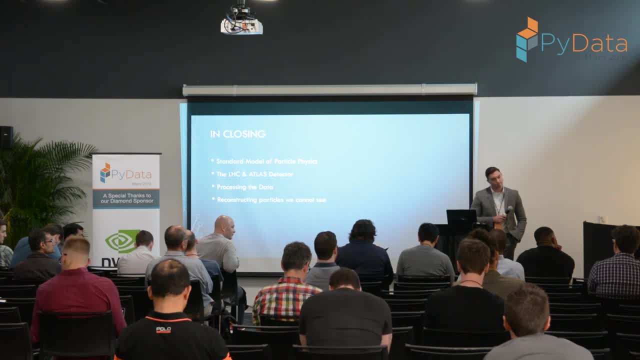 and then using machine learning to kind of sift through everything. Yeah, I'll be honest, How the Monte Carlo model works, although data itself is generated, I don't know much about. Um, That kind of gets past me. And then we were using a lot of uh. 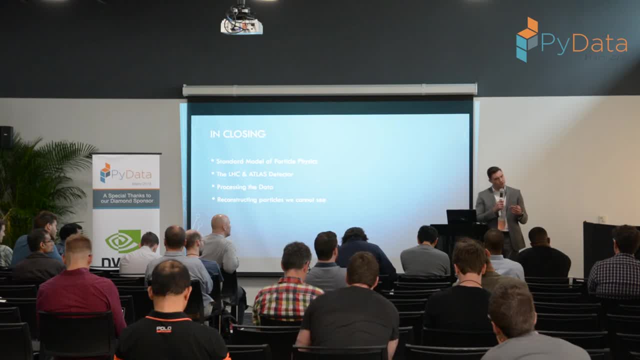 scientific data analysis framework called Root, Um, Which has a strange name because, like Root means other things too, But uh, Anyway, we used Root and C++ a lot Recently, though Python's, of course blown up. 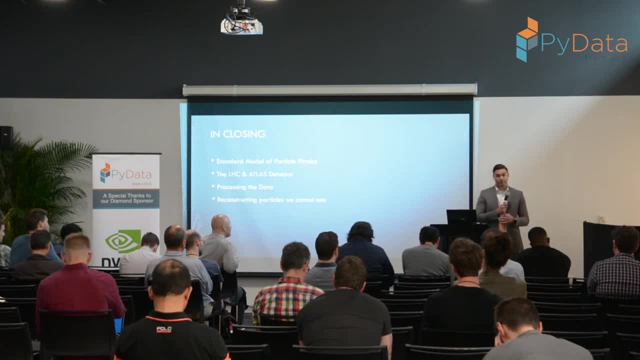 Uh, A lot more of the analysis is happening with that, But Root is that package And we can talk more about that. I can share links that way. Did I accurately answer your question, Or did I answer your question To some extent? 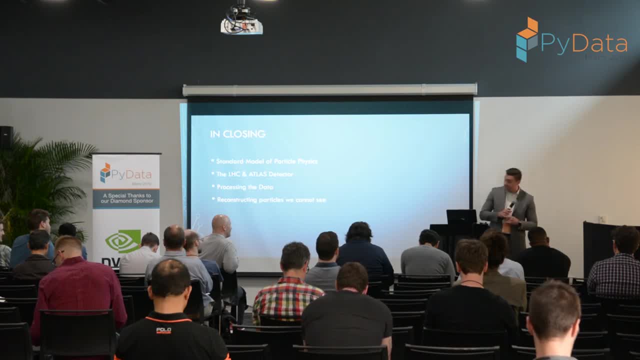 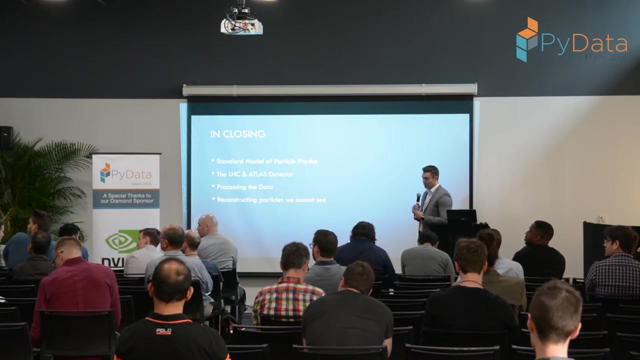 The answer is: I don't know. Yeah, Fair Fair. Any more questions? Sorry, You'd mentioned that. uh, you cut out some of the data to make. Yeah, What percentage of the total data set was cut out? Gosh, 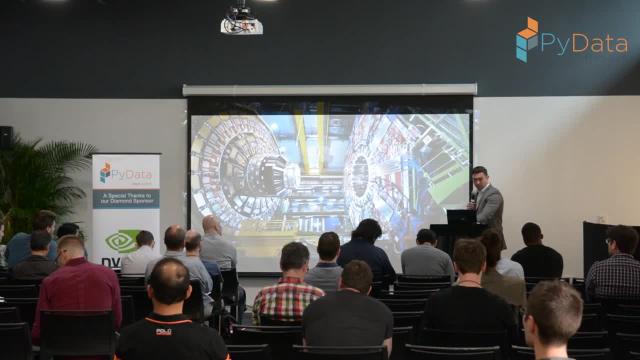 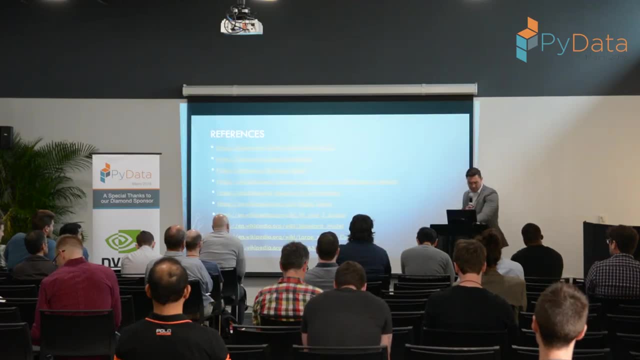 Most of it. Um, Well, let me So, In case you guys are actually gonna be like this guy doesn't know shit. Excuse my language. Uh, I appended an old uh, An old talk to the back of this. 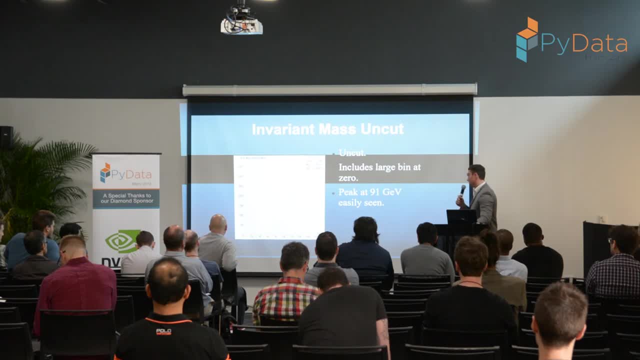 So let's see. This is what the data looks like without cuts. Yeah Well, so it says uncut, but it's not fully uncut, because some data, Some data is cut at like a physical level, like back at CERN. 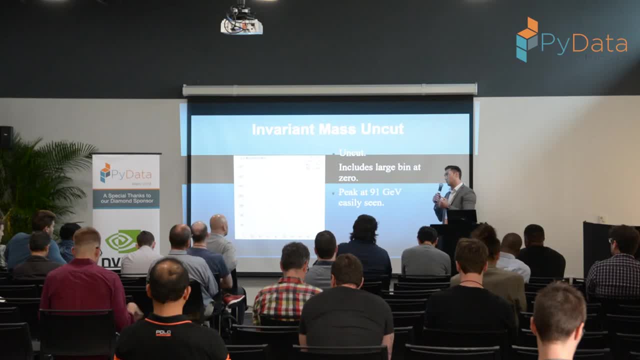 and I don't believe the data that would've been generated. They wouldn't. They wouldn't pass to us anything. If there's, uh, only one in 10,000 of those original like events that come through, they wouldn't. 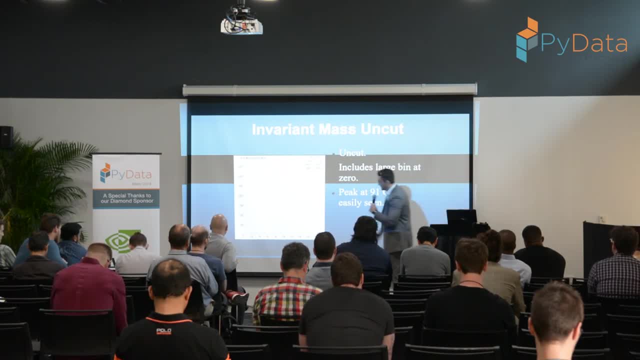 What I'm saying is, I don't know how to. I don't know how to say this correctly, so I'm gonna stop that. But if you see this, This is that first bucket where most of the events, or many of the events- 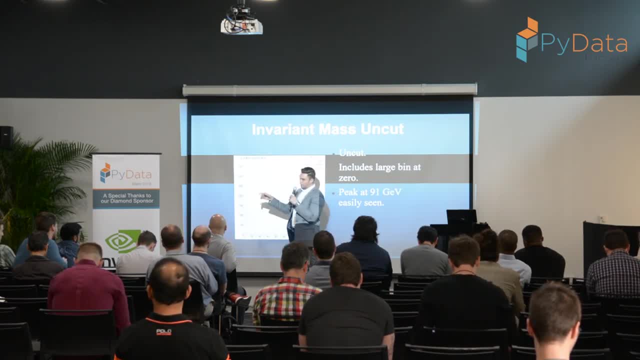 are events we don't care about. I just don't know whether many of these are at Done at that physical level when they choose one out of 10,000, or at the like software level where it's one event out of every 100.. 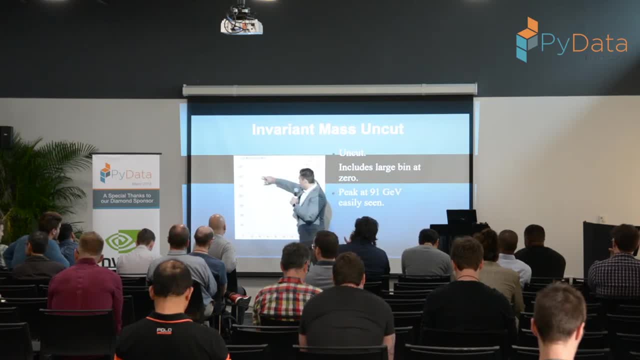 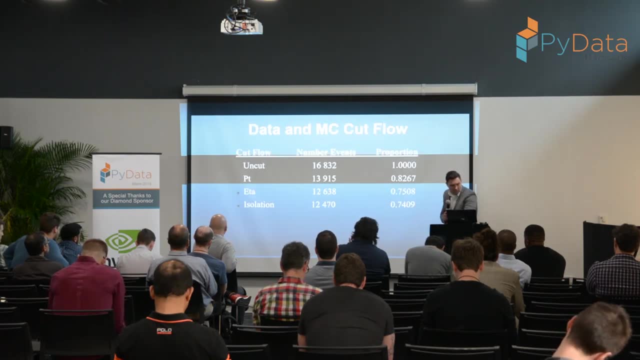 Does that make sense? So this bucket you. That's the first thing you cut out. The Let's see here Now. these are the different, These are the different cuts you make on your data. This is momentum, So 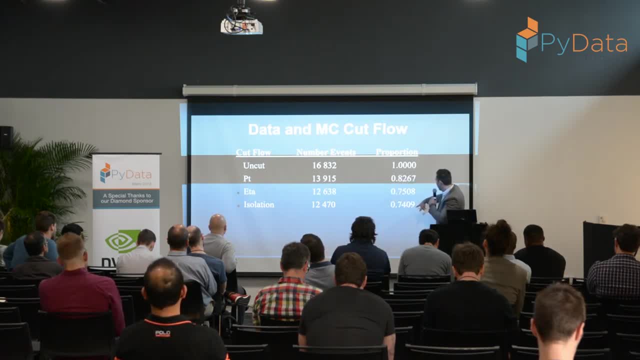 Oh, there you go. Ah, I guess at the end. by the way, you have 74%, I guess. yeah, I forgot. So yeah, you have about 70. 74% from from this particular run. 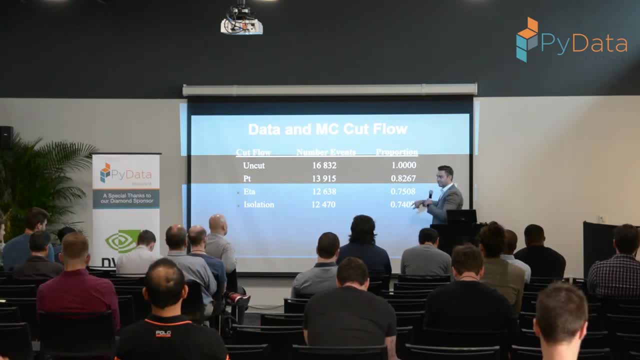 But I don't know if that's. I don't know if that's just this particular case or if that's the average. Does that make sense? So is that 74% data thrown away or kept Kept? Thank you, Yeah. 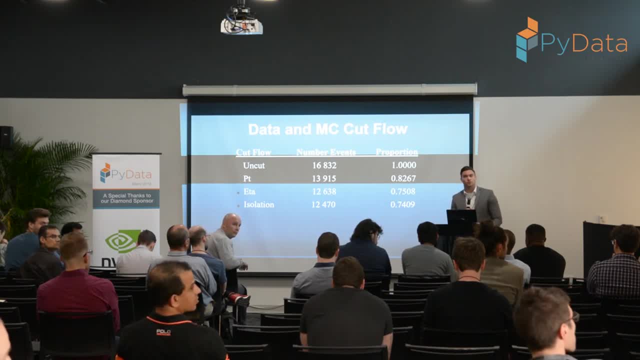 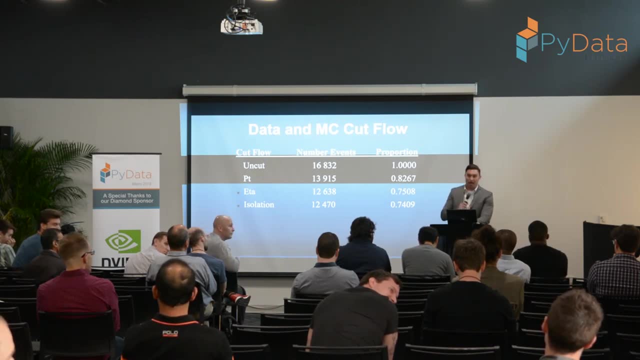 Sorry, We got one over here. Hi, thanks so much. You were mentioning something about working with Markov models in the intro of your talk- The Markov models. if you could speak a little bit about that, Sure, I actually. 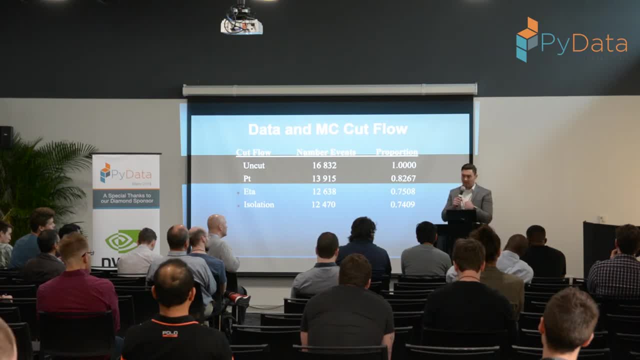 I didn't really work with like Markov processes or anything like that, It was Monte Carlo-generated data. Sorry, Not really, Not really. It's not. I wish, I wish I could, But yeah, I did. 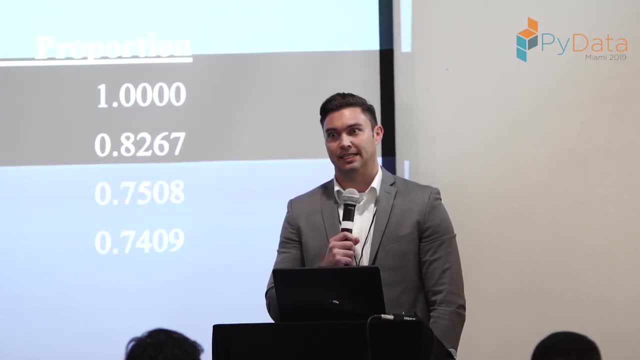 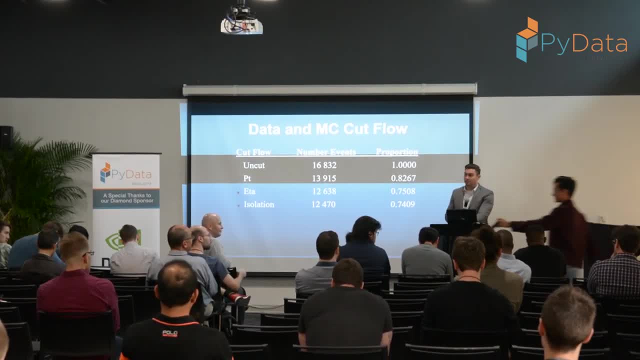 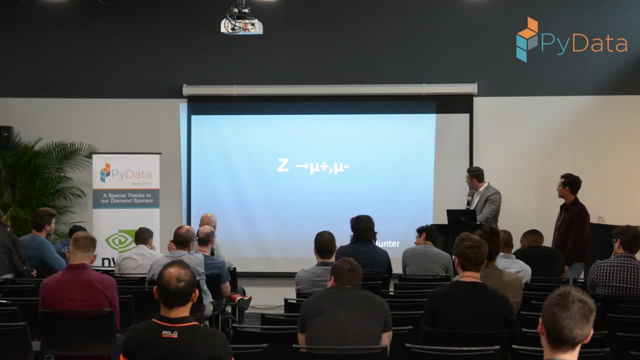 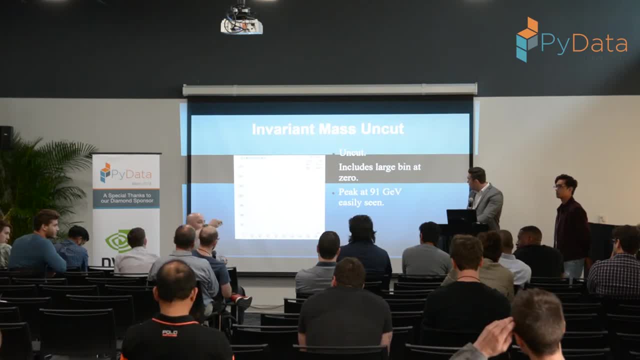 So yeah, So yeah, Okay, Okay, Okay. So now that you've kind of tried the graph where you had cut out a bunch of the data, Oh-oh, Sorry, Yeah, No problem, So yeah. 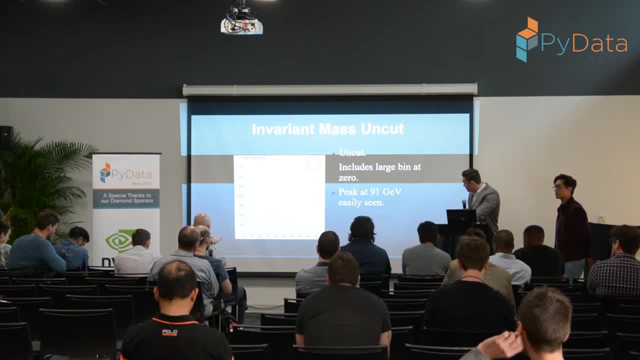 This one and you had the zoomed-in one where you could see the peak more clearly. You don't need to go to that. Okay, So I might have missed this. You might have explained it and I might have missed it. 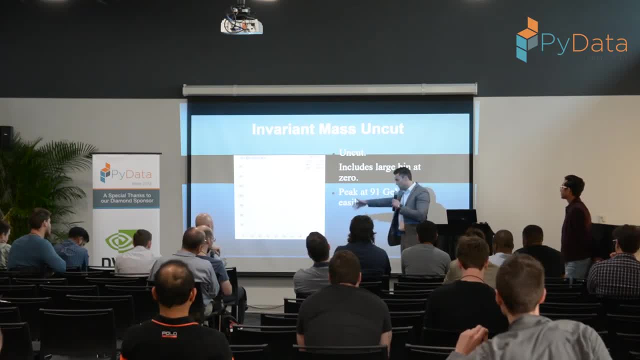 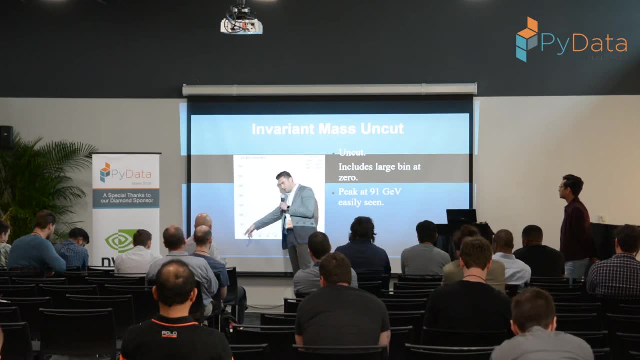 But what did you interpret distribution? there are small buckets and many, many of the events fell on this zero or I don't know if they classify non-events as negative one, I don't know if they have a special categorization, but 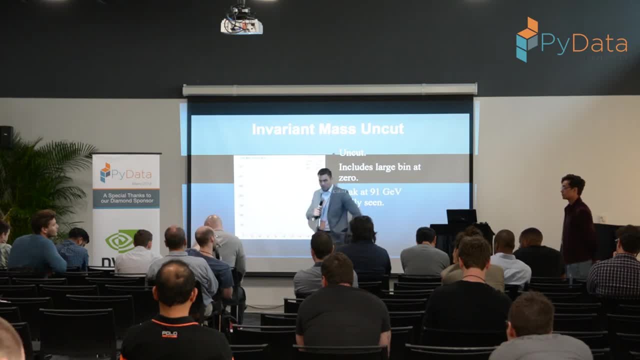 I'm trying to. I guess I'm trying to ask: did this prove something that you were setting out to prove And I missed what it was showing you? Yeah, So when you're trying to match the experimental data with what your theory says, you want. 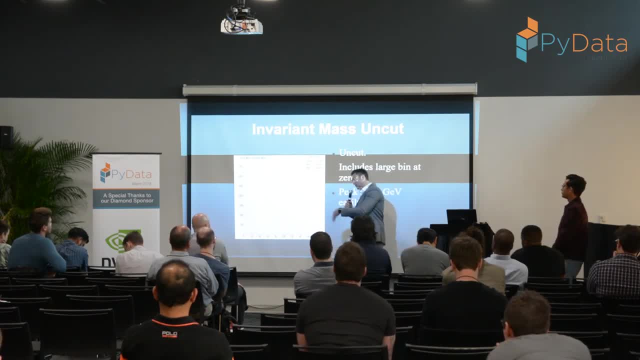 to have your software ready for what does our theory say? What does that kind of curve look like from the theoretical perspective? Because if you need to generate this line and then you have data that overlaps it, if I end up getting an experimental curve that is over here, well then this line's wrong. 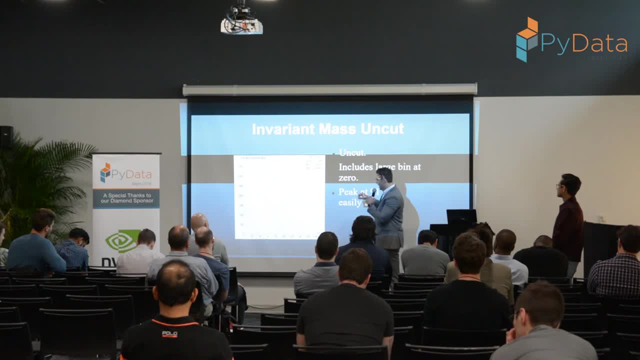 And a lot of the work at the time. So this is back in 2010.. Yeah, A lot of the work at that time was more on the theory side and not on the experimental side, because it wasn't fully up and running until years later. 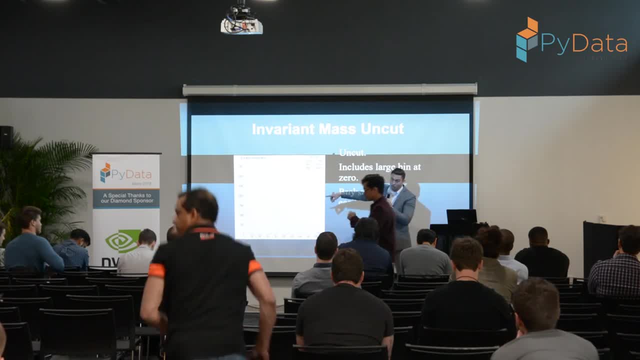 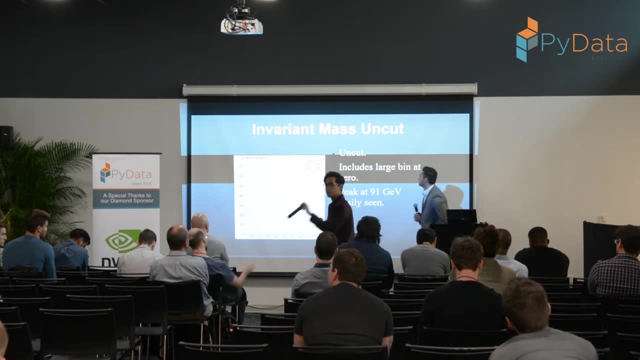 Hmm, Okay, Yeah, I interpret it as very low energy events. Okay, Thanks. One final question: Anyone wants Going twice? All right, We're good. Thanks everyone. Thank you guys.